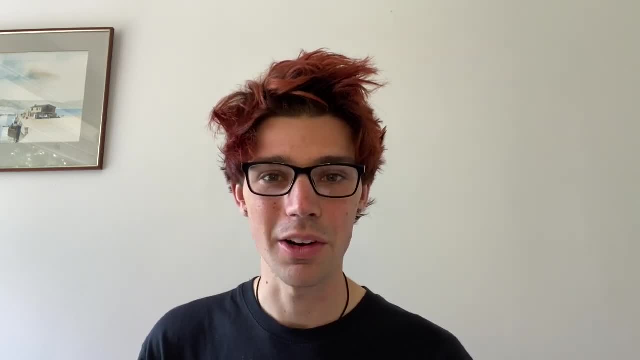 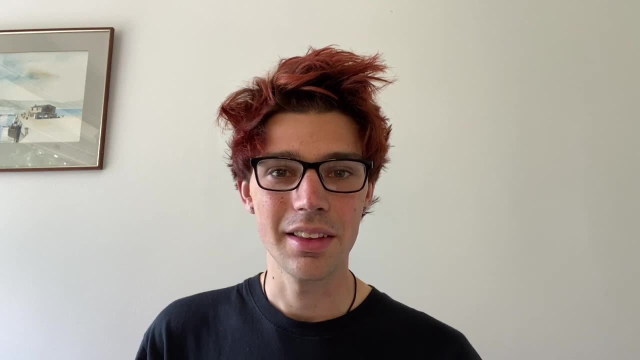 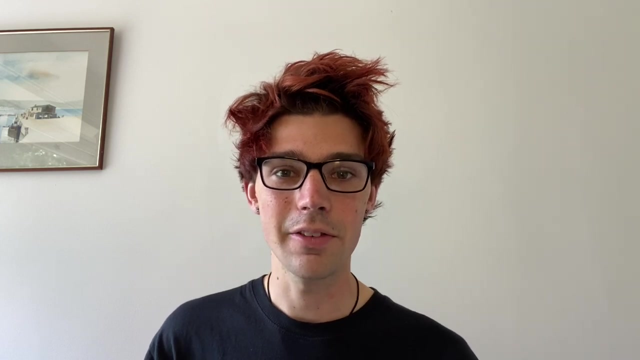 matter. In today's video, I'm going to talk about one of these new states of matter: the Bose-Einstein condensate. Now, this is a particularly weird state of matter because it's very hard to imagine and it's a highly quantum effect which is only visible at very, very, very specific conditions. These conditions are that it can only happen with bosons and also the temperatures must be incredibly low, like we're talking a few degrees above absolute zero. They can also only happen at very low densities, something like a millionth of the density of normal air. 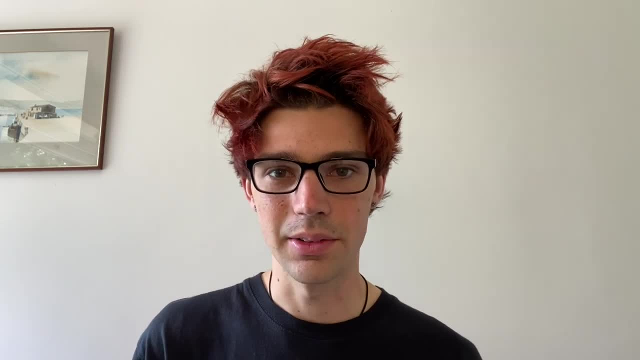 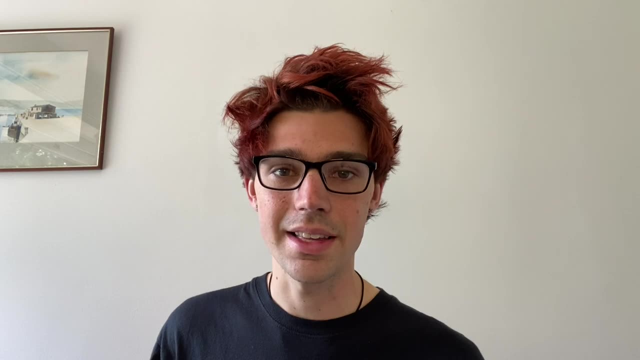 But how do these gases form Bose-Einstein condensation? Well, we're going to be using some of the knowledge in the previous video, particularly looking at the Bose-Einstein distribution, and we're going to be using that to see how we can derive this effect that we observe. 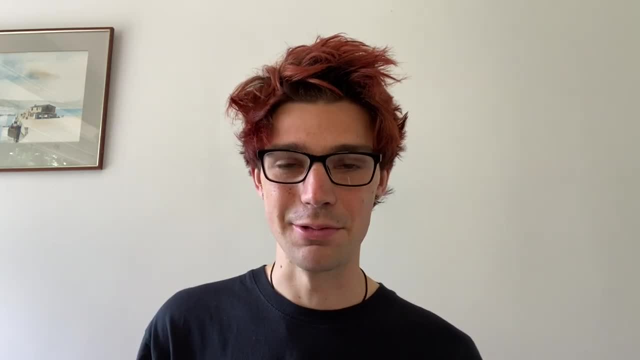 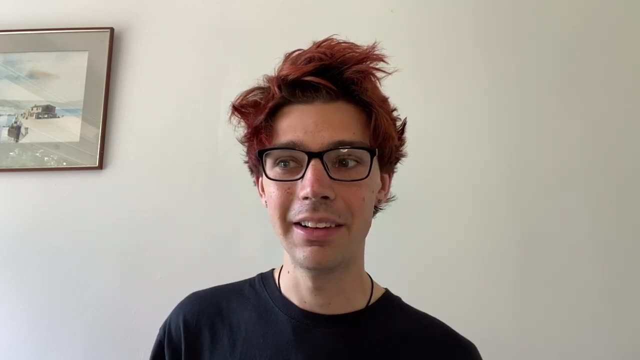 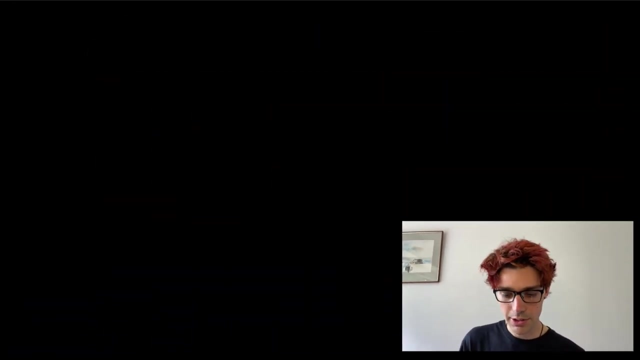 at very, very low temperatures And, believe me, this effect is really cool. It's like quantum mechanics, but happening on a macroscopic, everyday scale. It allows you to see wave functions, So without further ado, let's jump into it. So in the previous video, we derived the 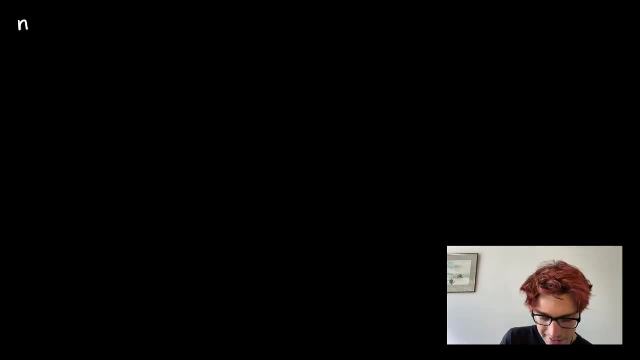 Bose-Einstein distribution and that we said that the average occupancy of a state k, of a single particle state k, is equal to one divided by e, to the epsilon minus mu over kbt minus one, And this was the Bose-Einstein distribution. 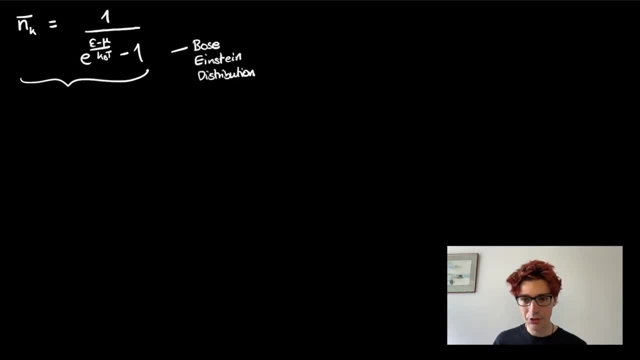 And basically it's telling you how likely it is for a particle to occupy a state given a certain temperature. So if we remember the Boltzmann distribution, it basically said that particles are more likely to be in lower energy states and it was kind of governed by the sort of exponential. 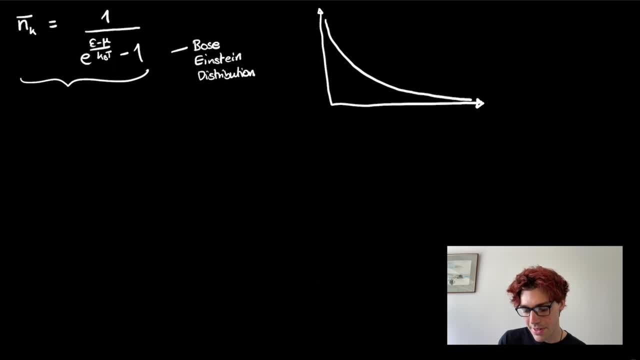 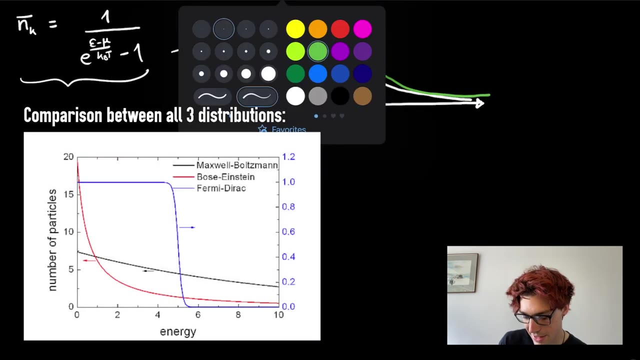 function right there, But the Bose-Einstein distribution is very similar. So if we plot the Bose-Einstein distribution it's very similar to the Bose-Einstein distribution for large energies, but at small energies it differs somewhat. So the two curves converge at large energies, but for small energies you find that there is a 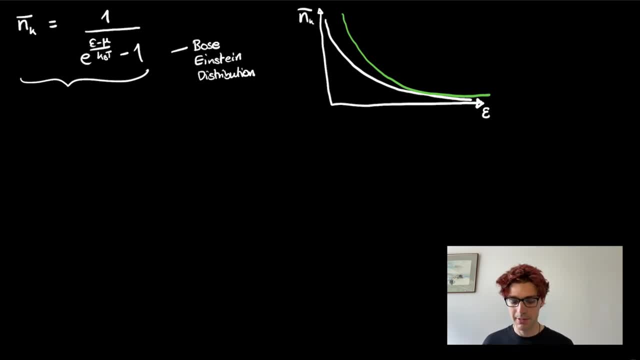 significant difference in the average occupancy right there, And this is coming from the quantum mechanical effect that happen when you get into this regime of low temperatures and densities that are on the order of the thermal wavelength which we talked a little bit about in the previous video. So I first want to 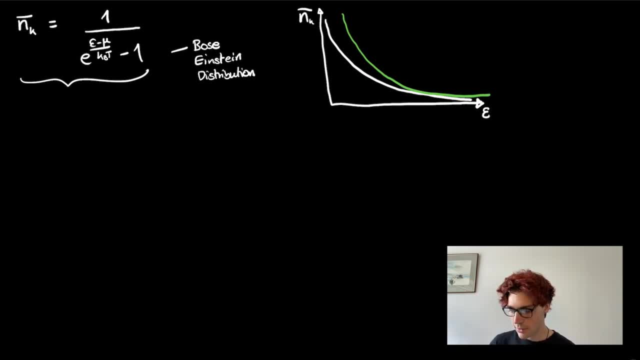 ask the question: what is the total particle number determined by? So if we imagine, like our very classic kind of box of box of gas, in this case it'll be a box of bosons. So I'm just gonna draw a box which has a certain number of bosons. 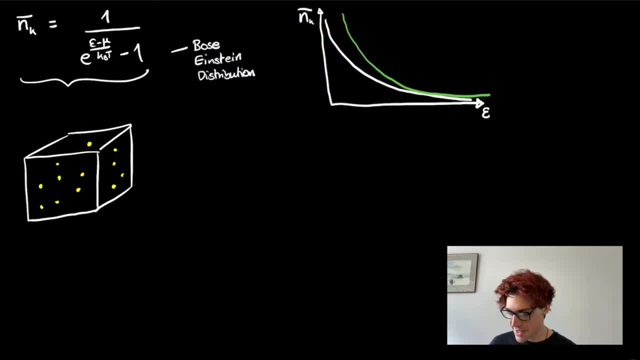 Now, if you remember our thermodynamic properties, we know that the box has a temperature T and it also has a certain chemical potential, because we're in the grand canonical ensemble where particles are free to flow in and out. It has a chemical potential of mu right there. So 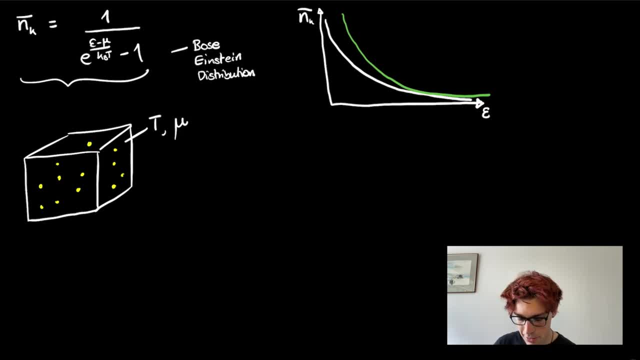 what determines this total number of particles? Well, we can calculate the total number of particles by simply summing over the average occupancy of each state. So if we look at the total number of particles, we can calculate the total number of particles by simply summing over the average occupancy of each state. So if we 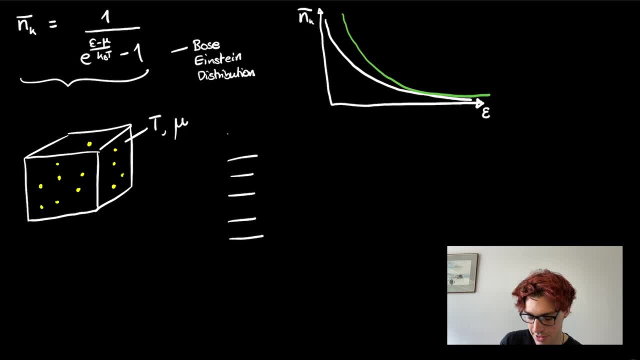 go through all of our states right here, which I've drawn as kind of like rungs on a ladder. then we can just sum up the total number of particles on each state So we can see: there's 1 in there, there's 2 in there. We've done this a few times before, so we can just obtain the total number of particles just by. 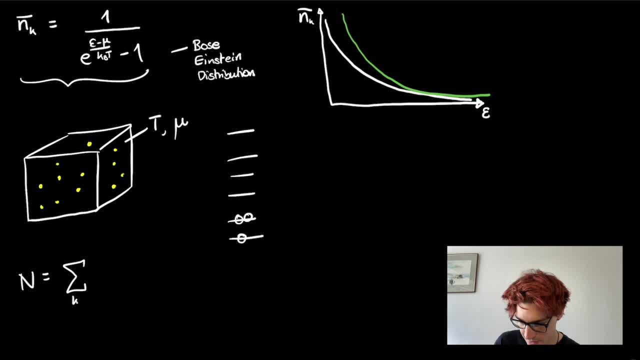 summing up overall the states, which I'm just gonna call K, the average number of particles in each state, Because of course it's going to fluctuate, because of course no particle is going to stay on its particular state. It's not going to be in the same state all the time, but each state is going to have an. 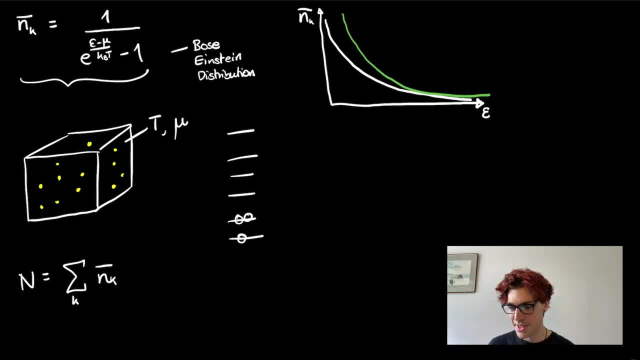 average number of particles occupying it. So if we sum over all these average particle occupancies, then we're going to obtain the total number of particles in the gas. So what are we going to do? Well, we're going to sum over the states. and what is this average occupancy? Well, that's just. 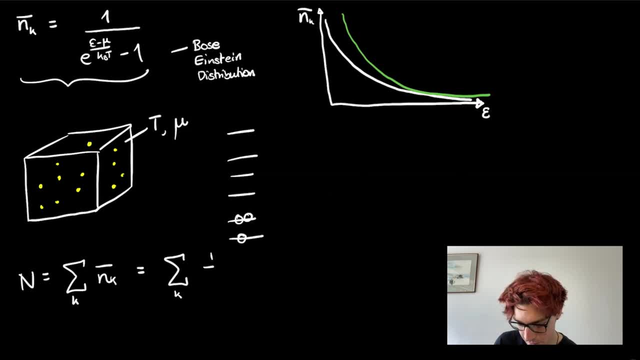 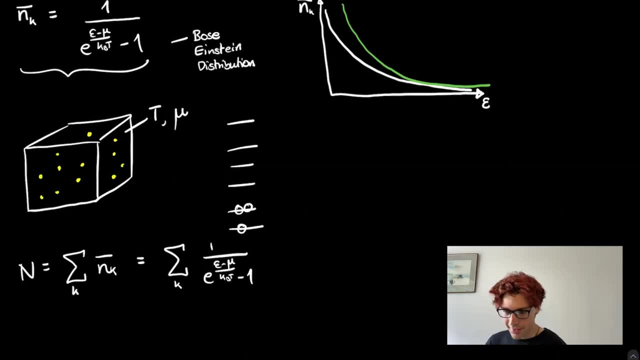 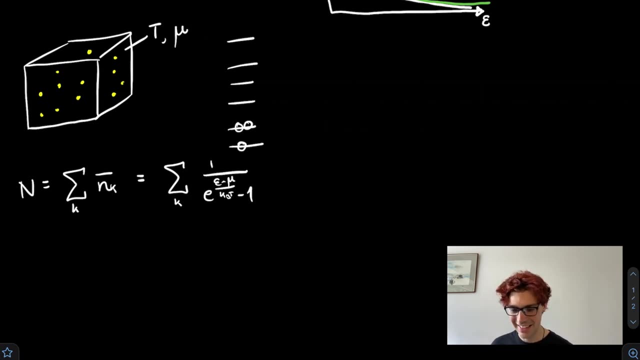 suppose Einstein distribution 1 over e to the minus epsilon, minus mu over k, B, T minus 1.. Now, we're talking about this a lot in theory, but in reality are we really going to sit here and count the number of particles in each ladder? because that is, let's face it, that's impossible. 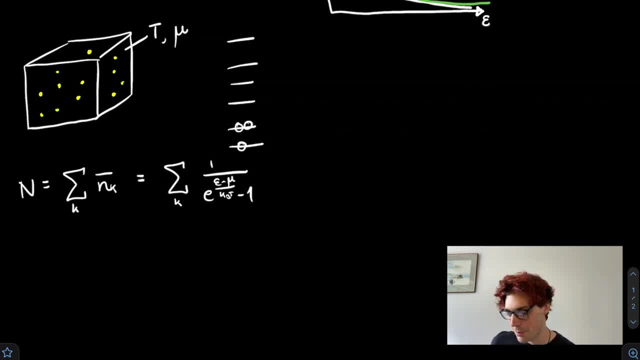 So we're going to have to do some kind of approximation. Now, what we often imagine is that we have a value of one to the minus epsilon, minus mu, over e to the minus epsilon. do we did this in the density of states derivation, but what we are going to do with this is we are 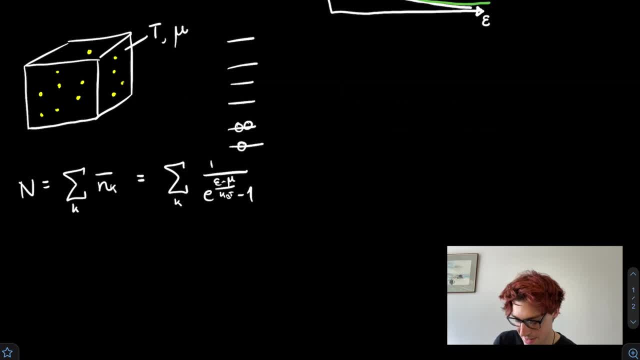 going to convert this: rather than being a sum over discrete states, we are going to convert this into an integral over sort of a continuous set of states. Now, this is an approximation because obviously states are not technically continuous, they are discrete because of quantum mechanics. 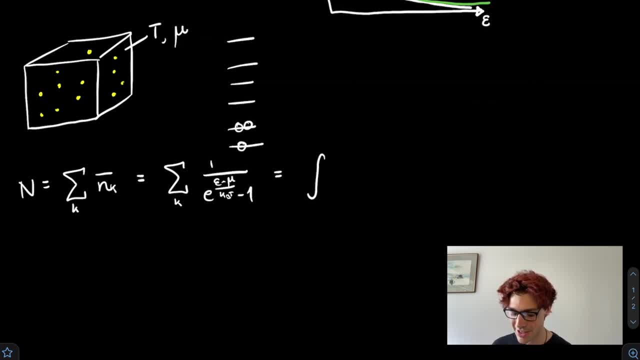 that's basically what quantum mechanics is saying. you can only have discrete energy levels, but since there is so many, you might as well treat them as continuous. It's like having a sort of hair comb which the blades are so so, so, so fine together that it might as well just 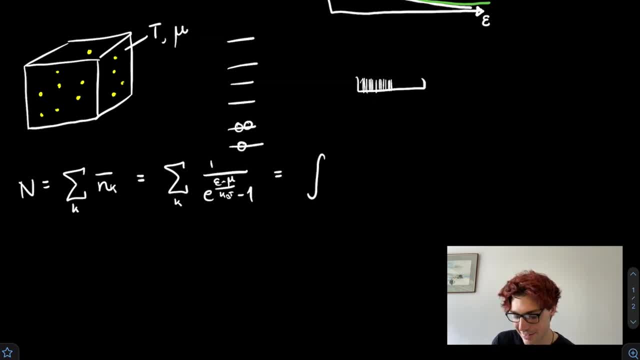 be a smooth metal. basically, that's kind of a good analogy of looking at it. So we're going to be doing an integral over all operators, the states. but of course, when we derive the density of states, we convert it from integrating over states to integrating over energies, which is much, much, much. 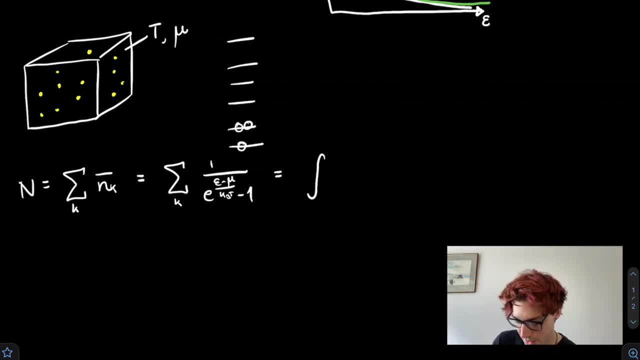 easier to do. So what we're actually going to do is we're going to integrate over energies. so we're going to go from zero to potentially infinite energies and we're going to integrate this function right here. Of course, we have to also include the density of states function, because there are going. 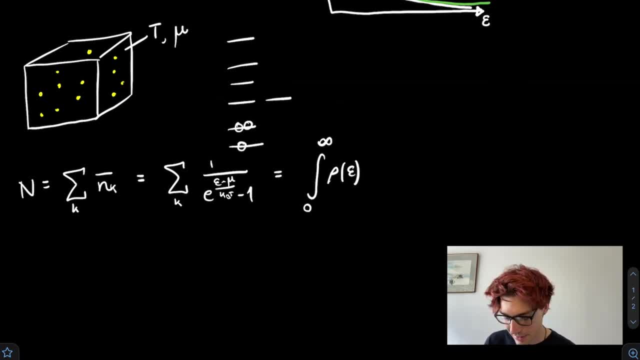 to be multiple states at the same energy. so this will be like in a discrete example like this. so we obviously have to count all four states right here, So there's our density of states, and then we're going to multiply this by the Bose-Einstein distribution right here, and then this is all going to be. 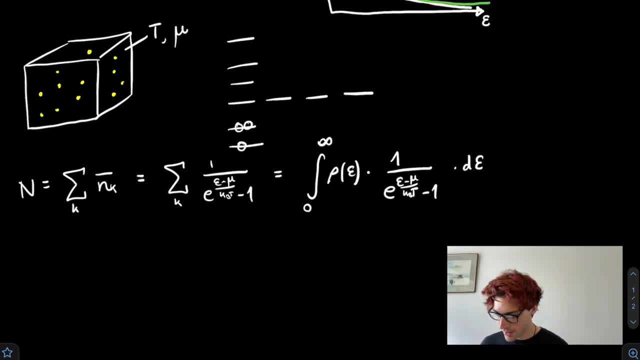 integrated with respect to epsilon. So this is our integral right here. This is going to help us work out the total number of particles in this box. In this case, it's going to be the total number of bosons. This is a general formula that you can use to work out the total number. 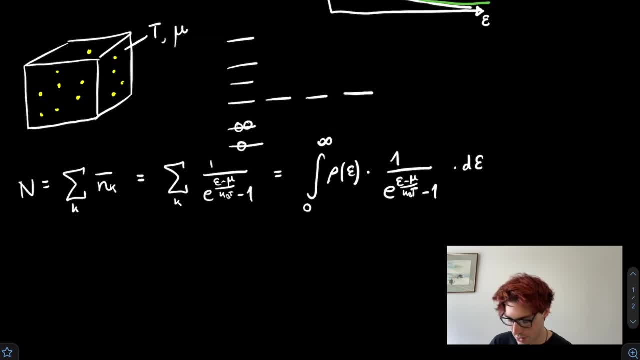 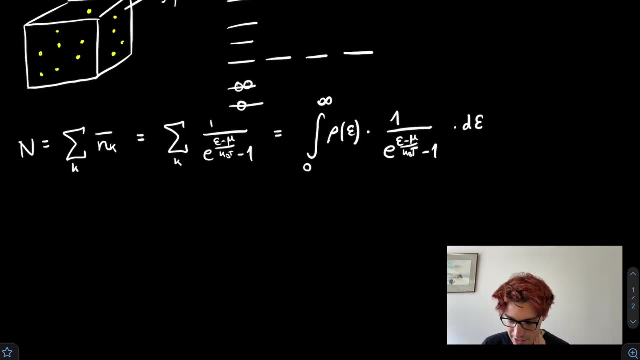 of bosons in a system. This is generally how you do it: You multiply density of states by Bose distribution and then integrate that all over energies. So what did we say? the density of states was. Well, when we derive the density of states, we had to use the dispersion relation, which 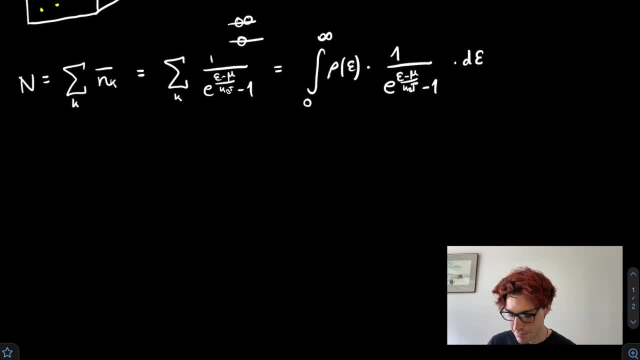 basically is the relationship between energy and momentum. Now this is, of course, going to be different depending on what type of bosons you're going to be working with. So for light, if you remember, the dispersion relation was: epsilon is equal to momentum simply multiplied by the speed of light. That 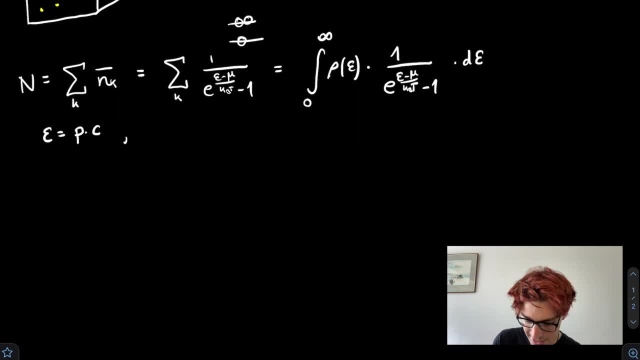 was a linear dispersion, But for massive particles, which are particles that have mass, then the dispersion relation was p squared over 2m, which is literally just half mv squared, but written in terms of momentum. Now, in this case, we're going to be dealing with bosons which have a mass. 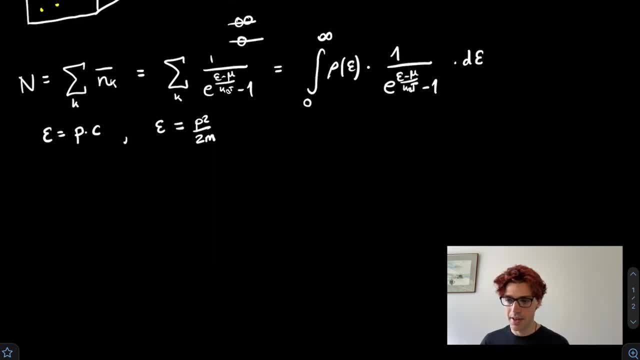 And this is typically what makes up the Bose-Einstein condensates. Now, it's interesting to consider at this point: Not all bosons can have the ability to form a Bose-Einstein condensate. Now, this is a mathematical thing. When we actually reach the part of the 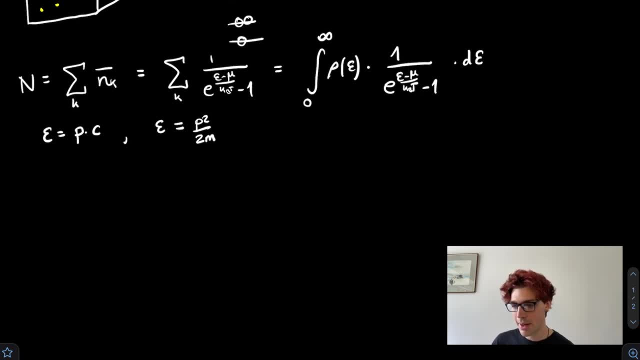 derivation which determines whether a particle can become a Bose-Einstein condensate, then I will point it out, But for now just note that massive particles. we are going to be using the dispersion relation for massive particles, which is this right here? So what was our density of states? 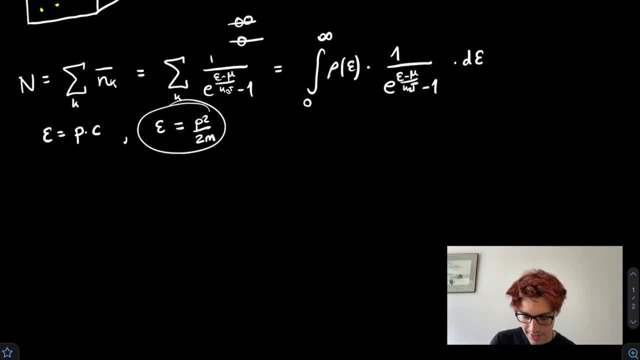 If we remember back to the video I did on density of states, then we found that the density of states for particles which had a mass was something a bit like this: You would have your energy along here and then the density of states would scale proportionally. 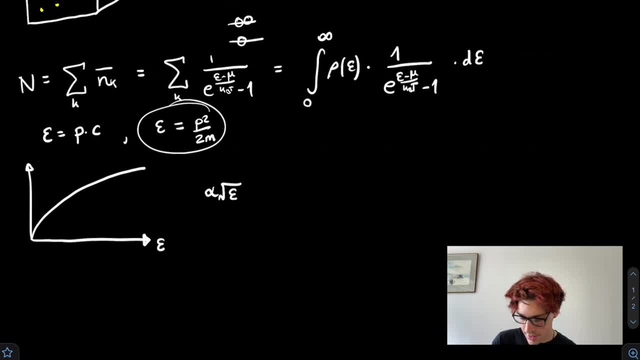 to the square root of the energy. So there are a whole bunch of other constants that were before in the prefactor, but basically the density of states would scale proportionally to the square root of energy, And for our purposes that's kind of all that matters. We don't really care about all these. 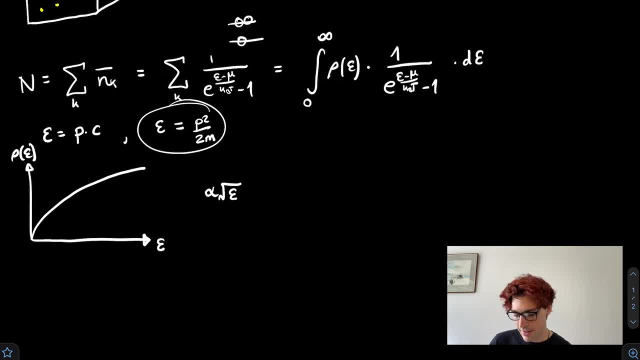 constants a huge amount. We're only interested in pretty much how the density of states scales with energy. So what I'm going to write is: I'm going to write that this integral right here, I'll write it over here. So this is going to be equal to: 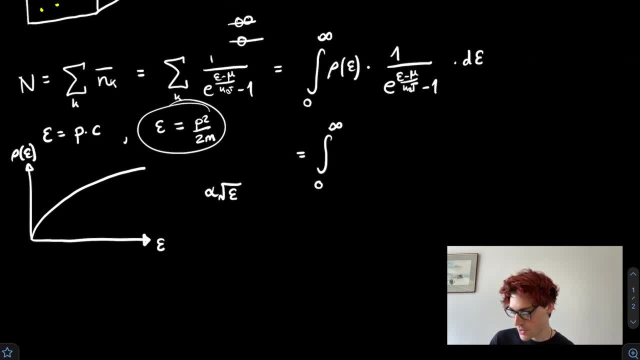 So this is going to be equal to The density of states, which we said was proportional to the square root of energy. So what we're going to write is we're going to write a bunch of constants, which is basically all these constants, which includes mass, h, bar, pi or whatever. 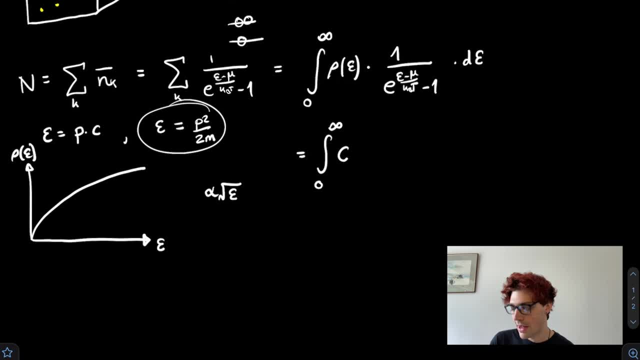 And we also said that the density of states includes a volume term as well. Now, normally, the volume term would be treated as a constant. However, with Bose-Einstein condensation, we're going to be talking about densities a lot, So we're actually going to write the volume term right here. 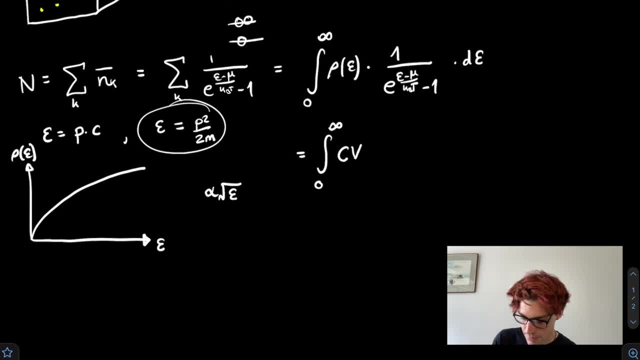 And then we're going to multiply this, of course, by the square root of epsilon. So that is basically our density of states term. right here, In fact, more explicitly, I'll write out what the density of states actually is. So it's c multiplied by v, multiplied by root epsilon. 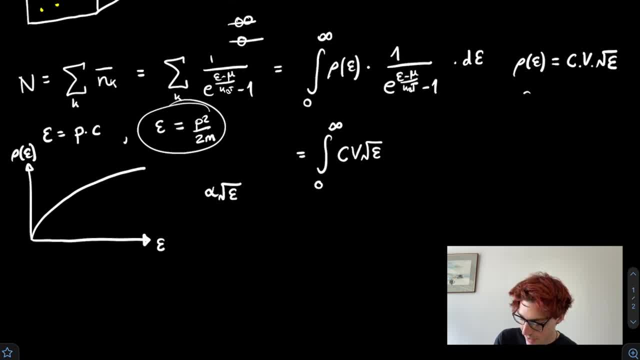 And c I have defined So it's c multiplied by v, multiplied by root epsilon And c I have defined So it's c multiplied by v, multiplied by root epsilon And c I have defined So it heres the density of states of particles whose density is four pi root 2 mass to the 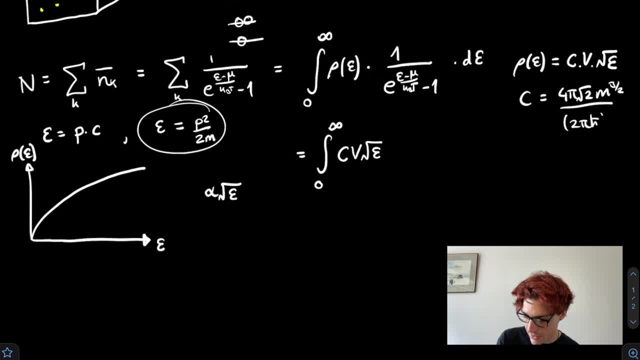 three over two over two. pi h, bar cubed. So this is the density of states for particles which had mass And basically the way I've written it is, I've factored all the constants into this term c, apart from the volume Which normally we would consider a constant. 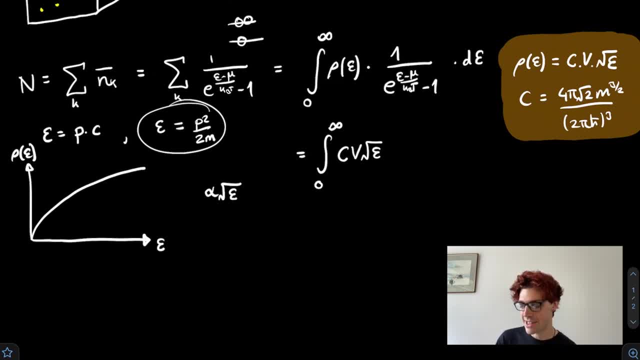 Normally we're only interested in how it compares, in how it scales with energy, But for this particular case we're leaving volume in the whisker, And so we bring that. so this is找 by maar, which is the settle of the walls which are 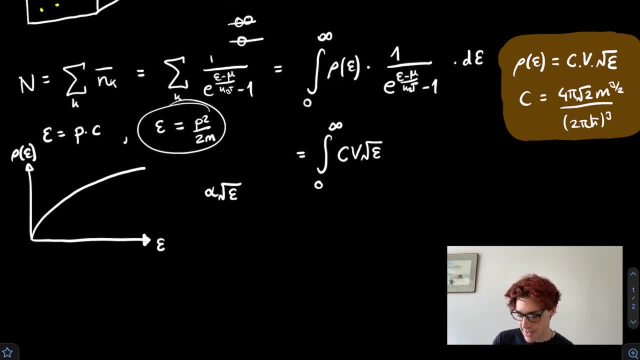 there. So that's the density of states. And then we're going to multiply this by the Bose-Einstein distribution, So e minus mu over kBT minus one integrated with respect to energy. Now this isn't a hugely easy integral to perform right away, So we need to think. 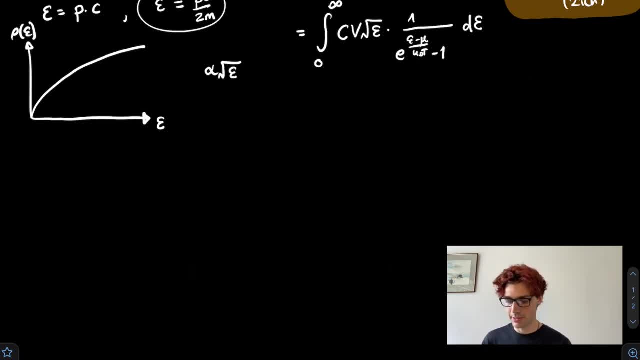 a little bit first, before we actually perform this integral. Now, the most problematic thing is this chemical potential. mu, right here Now. Bose-Einstein condensation basically only happens when the chemical potential reaches as close to zero as it can possibly get. We. 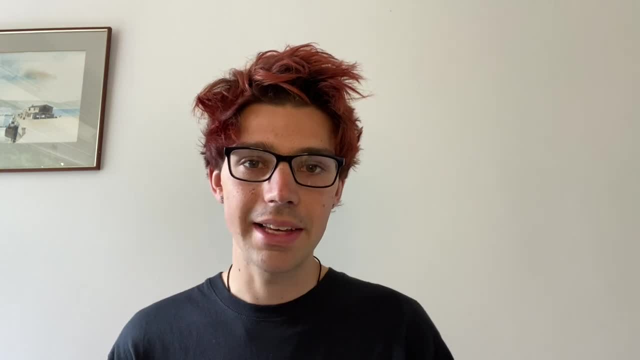 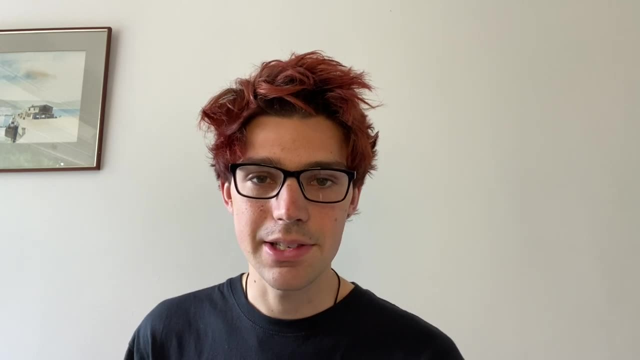 talked a little bit about how, in the dilute gas limit, the chemical potential is as close to zero as it can possibly get. So the chemical potential was very, very, very far away from zero. The further away from the chemical potential is to being from the thermal energy then 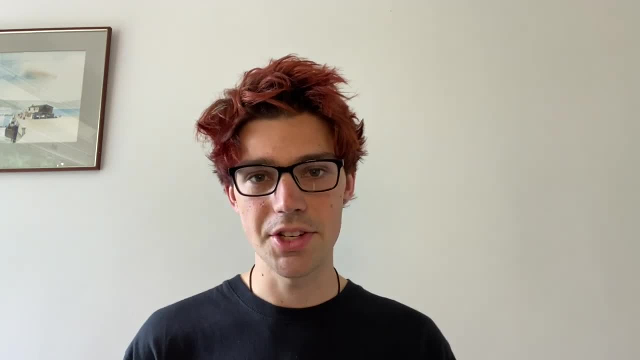 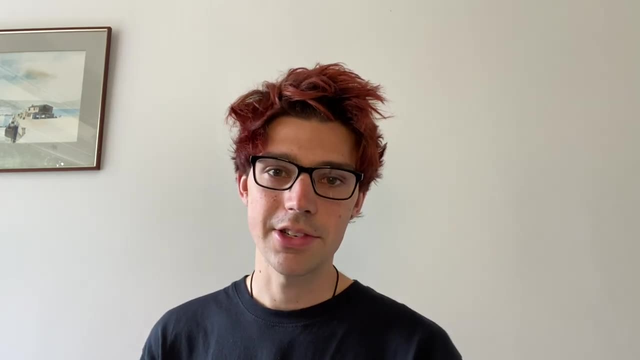 the more like a classical gas it behaves. But we're not in the classical regime, We're in the quantum regime. So we are going to consider the case where the chemical potential becomes very, very close to zero, asymptotically close to zero. So let me just draw a graph. 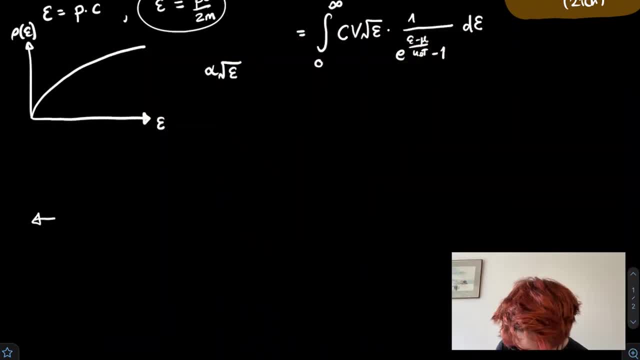 of this real quick, just to show you what I mean. So chemical potential, which of course we said was negative. So I'm going to draw a kind of reversed axis right here. So here's our chemical potential And then here's our total number of particles. Now for a gas, it's. 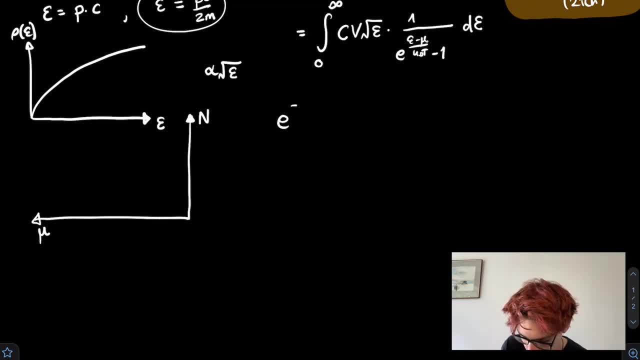 of course sort of equal to e to the minus mu or e to the plus mu over kB T, because of course mu is in itself negative. So we're going to get this reverse exponential curve. So this is the curve right here Now. this was of course in the classical regime, But 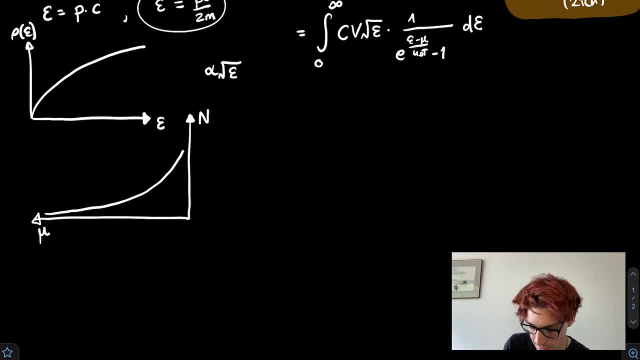 what's going to happen when mu gets very, very close to zero? Then we want to find out what happens at this critical point right here. What happens when mu- the chemical potential- equals zero. So this is basically what happens when we start getting the effects of Bose-Einstein. 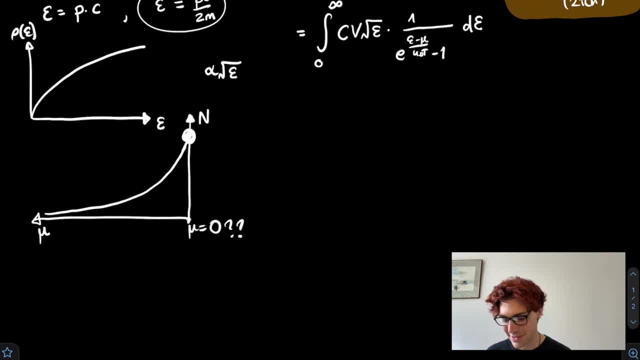 condensation. So, basically, the condition for Bose-Einstein condensation is that mu is equal to zero. So that's the thing you have to bear in mind: mu equals zero. So what we're going to now do is we're going to calculate the total number of particles. 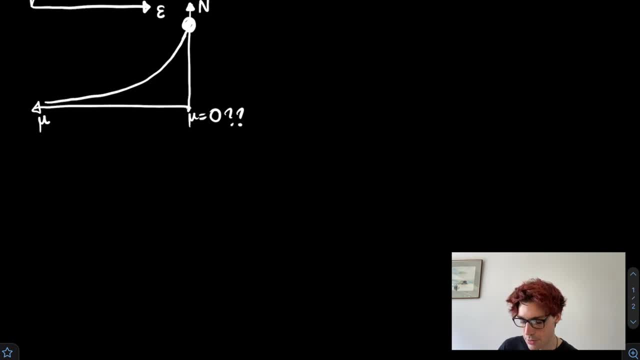 in the box, in this specific case of mu being equal to zero. And just to signify that this is a different quantity, I'm going to call this quantity n star Now. n before, just for comparison, was the total amount of particles in a box. 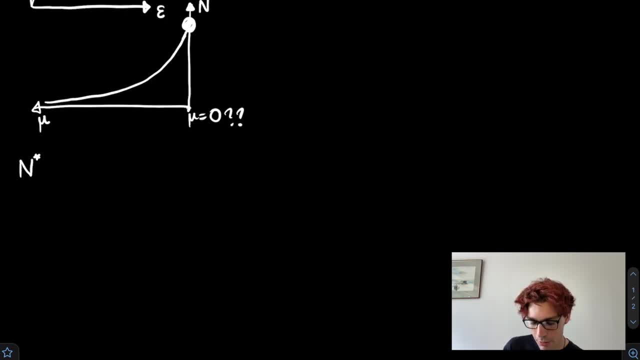 as a function of chemical potential and temperature. But now we're fixing chemical potential equal to zero. So now we are gonna try and find out the total number of particles in the box for zero chemical potential. So let's just go ahead and rewrite what we wrote. 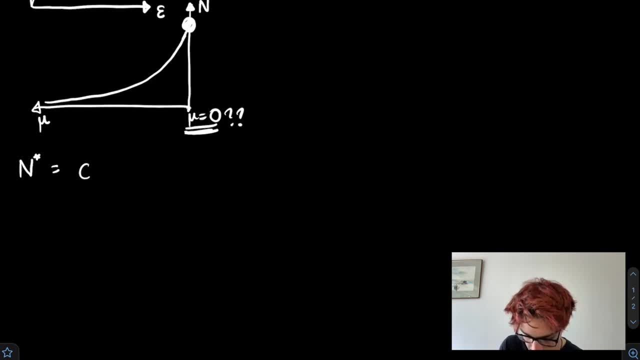 So we have Cv, which are actually constants, so I'm gonna factor them out. the front of the integral times, the integral between nought and infinity, of the square root of epsilon, all divided by e, to the epsilon minus mu, which is what we had before. 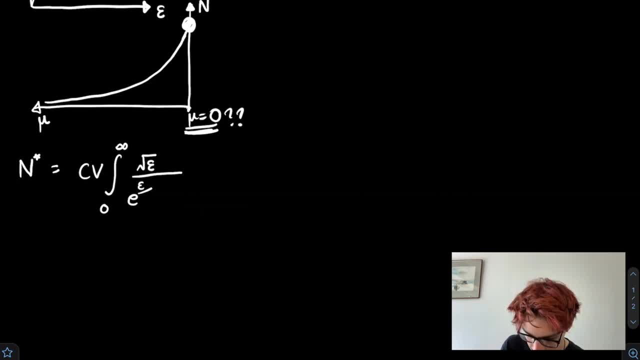 but of course mu is zero, so it's gonna be minus zero over kbt, minus one d epsilon. So now we have this integral which will enable us to find out the total number of particles in this box. So what we're gonna do? 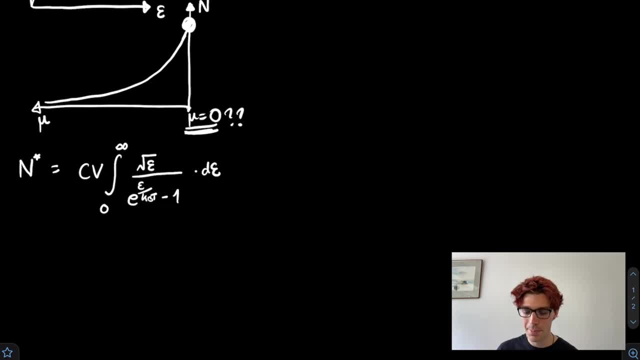 is. we're gonna have a look at this integral and we're gonna see what happens to this integral near the limits. Now, this is a trick that often mathematicians like to use. You inspect the value of the integral near both the lower limit and the upper limit. 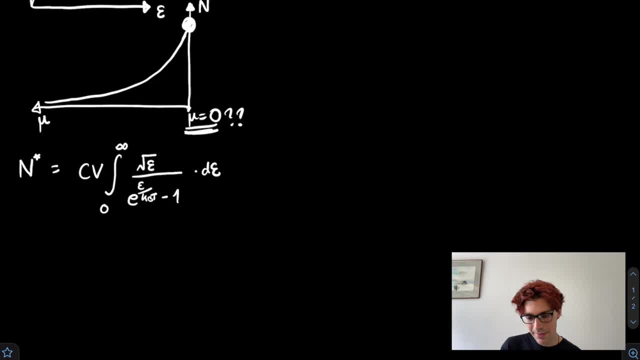 And if it looks like it's not diverging to infinity, then basically that tells you that you have that, this is mathematically sound or okay, And in our case, it tells us that we can get those Einstein. and that tells us that we can get those Einstein. 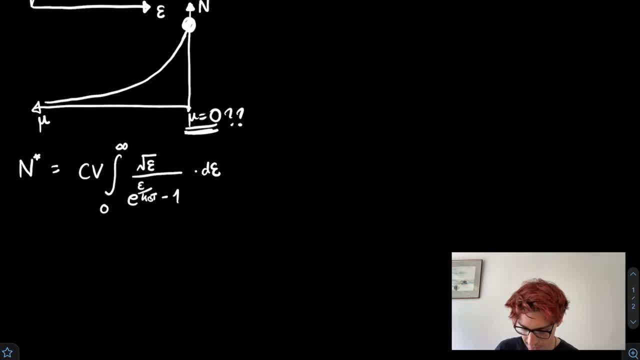 condensation. What I'm gonna do is I'm gonna make the substitution that x is equal to epsilon over kbt. I will do a substitution very similar to this a lot of times. It's basically just a trick to kind of make the integral. 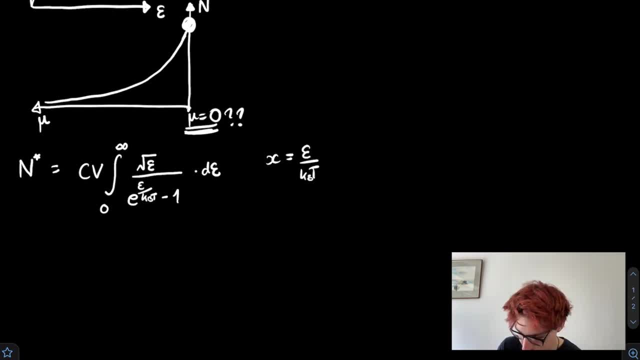 and the maths a little bit easier. And if we take a differential, you can see that dx is equal to d epsilon over kbt. You can see that dx is equal to d epsilon over kbt. So that's our substitution, right there. 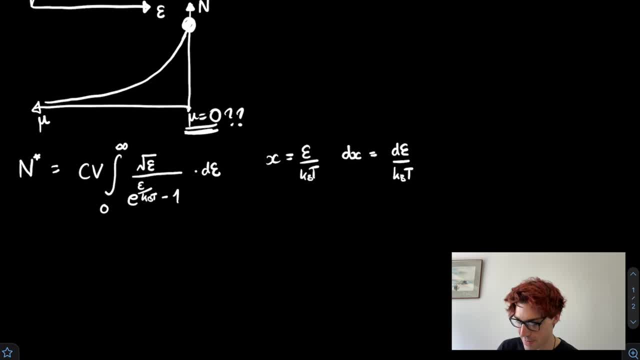 And now we're just gonna go ahead and replace all the epsilons with xs, right there. So n star is equal to cv multiplied by the integral. Again between naught and infinity, because x scales linearly with epsilon. So if epsilon goes between naught and infinity, 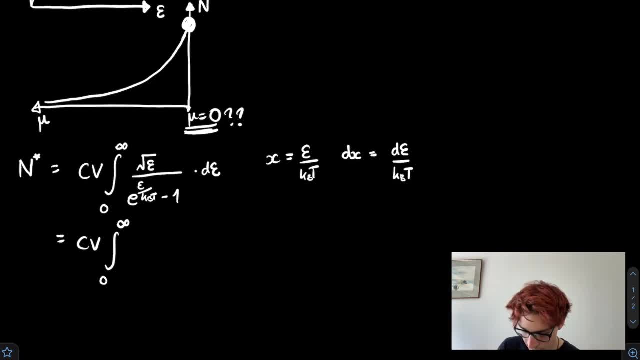 x will also go between naught and infinity. We're gonna have, instead of root epsilon, we're gonna have root ardent. And then we're gonna have, instead of root epsilon, We're gonna have: instead of root epsilon, we're going to have kB T x. Instead of writing the square root, I'm just going to write it as: 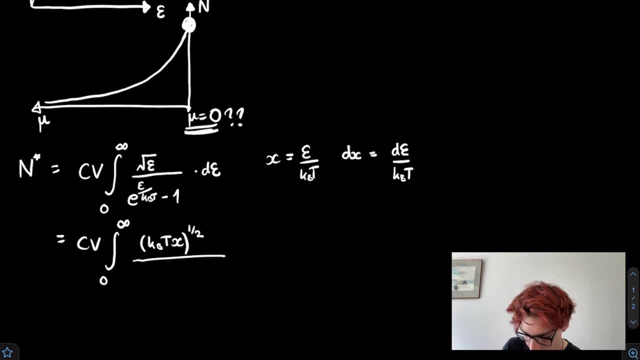 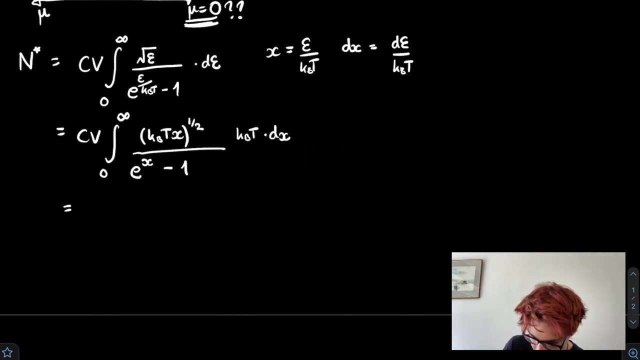 the power of half all divided by e, to the x minus one, And instead of d epsilon, we're going to have kB, T, dx And just to tidy it up a little bit, we're going to get c, v and we're going to. 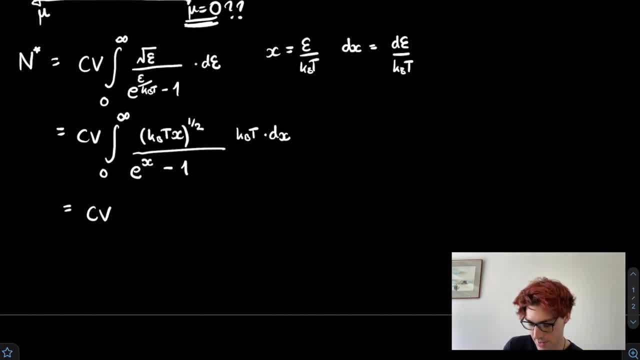 get these kB T terms, which were all constants, coming out the front of the integral And we can see that there's a kB T to the half right there and a kB T just as it is. So we're going to get kB T to the power of three halves out the front of the integral And then I'm going to integrate. 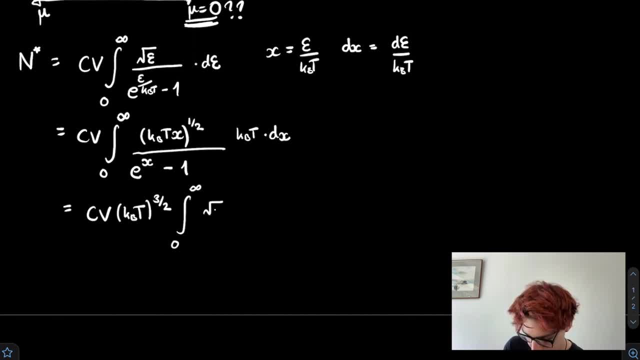 between naught and infinity. root x, because that's all that's left of this term. everything else has come up front, divided by e to the x, minus one, integrated with respect to x. So now let's have a look at this integral. 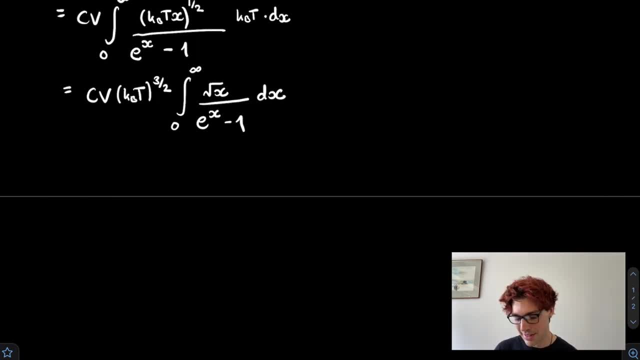 right here. Now that we've got it in a better form, we can have a look at this integral and see what's happening at the limiting cases. So, as x goes to infinity, what's going to happen to this integral? Well, whenever you have an exponential term, 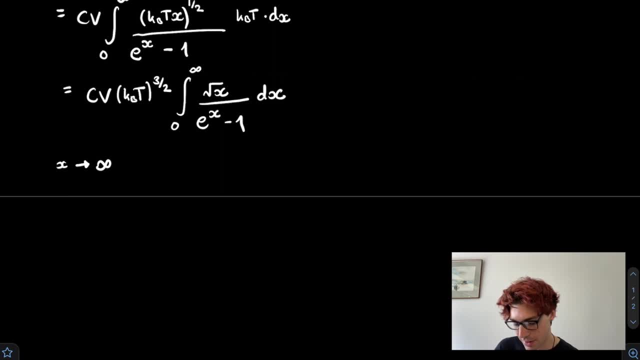 what's going to happen to this integral? Well, it's going to be a very domineering part of any mathematical expression because e- like if you graph e, then you get this very, very upward slope. Of course you're going to have other functions like x squared or x to the half. They're also 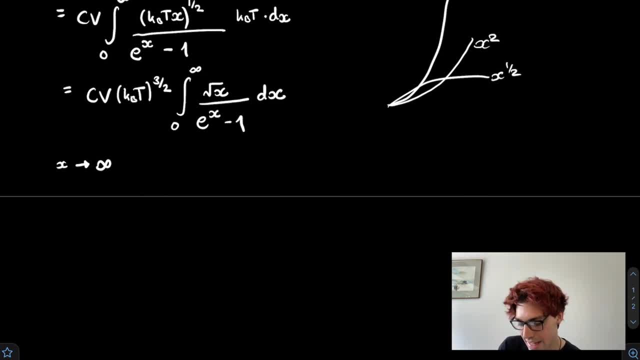 going to kind of play a part, but e to the x is the most domineering function. You can think of that as the thing that pretty much determines what happens in the limiting cases. It will kind of ride anything else. So, as x tends to infinity, e to the x is going to get very, very, very very. 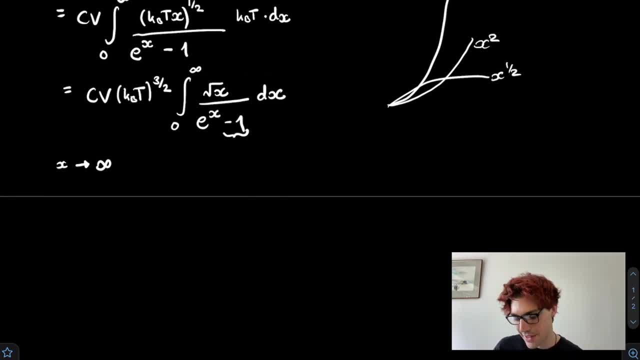 very big, And so this one, I think, like I said in the last video, isn't really going to matter. So basically, root x over e to the x minus one. this will basically become root x over e to the x for large x, And that is equal to root x, equal e to the. 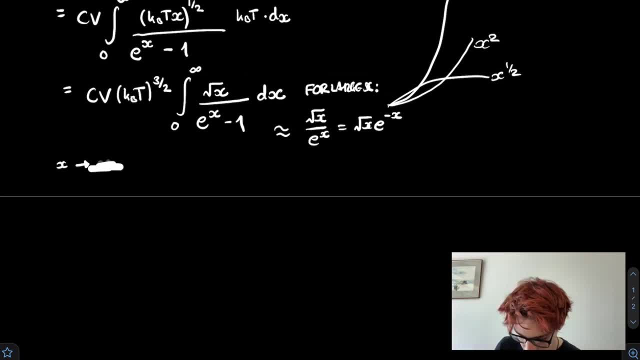 minus x just turning the exponential on its head. So what's going to happen to this integral root x e, to the minus x? Well, if x is large, then root x will be large. sure, but what did I say before? The domineering term of any product of functions is anything inside the exponent. 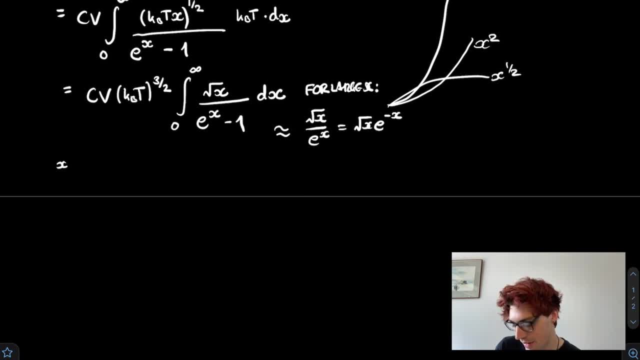 Now for large x, e to the minus, a very large number is basically zero, so it's as close to zero as you can get, and what that basically means is that for large x, when x gets really, really high, it becomes basic first of all. this basically becomes this, and you can clearly see that. 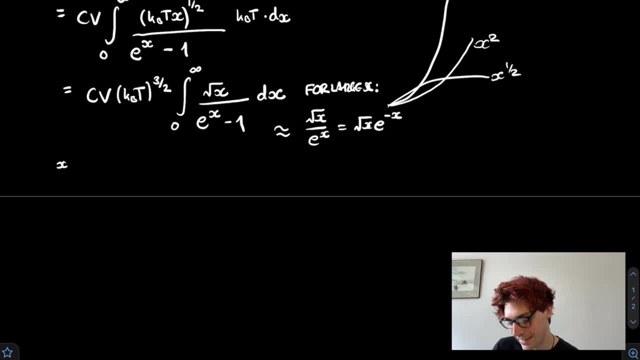 when x is large, then you can see that the this whole thing will basically become zero for large x. so this is only. this is kind of the upper limiting case. So that's kind of what we want. this is good. this means that you won't find that the number of 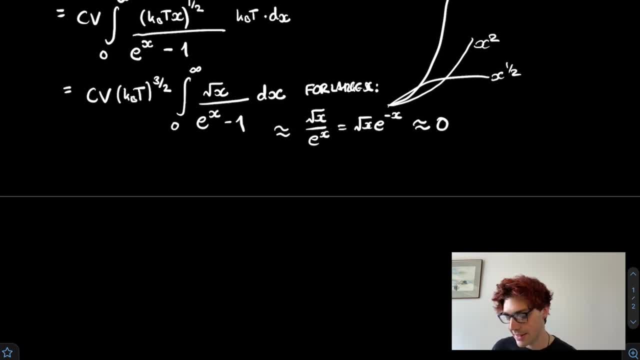 particles in the box will just increase drastically. it will converge to a certain point. so mathematically, this is fine. What about the other case? What about when x is very close to zero? So, as x is small, then what happens? It ties up to this equation right here. so you have root x over e to the x minus one. well, what we do? a. 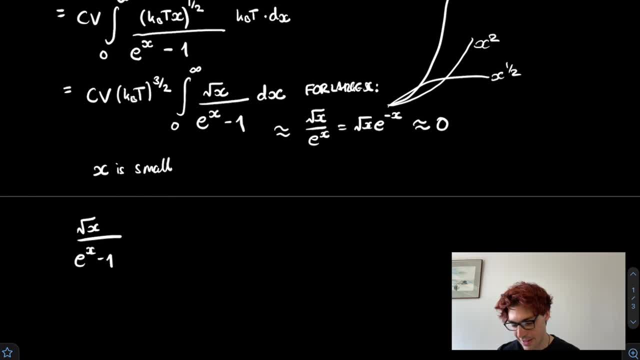 lot in maths is that if, if x is small, if the argument is small, what we can do is we can do an expansion. um, we can use the Taylor expansion just to approximate what it will be like for very small arguments. So e to the x vou small x is the之 sub. e to the x minus one forward versus x is equal. to put, uh, the spin on the Sammy situation just a little bit higher in your panel, very pretty safe és one that is a little bit more complex. I'm going to go over something on the side. I'm trying to do this one again, one to be same sort of for theOPI, as we say. so See, if x is less than 4, then you've got. 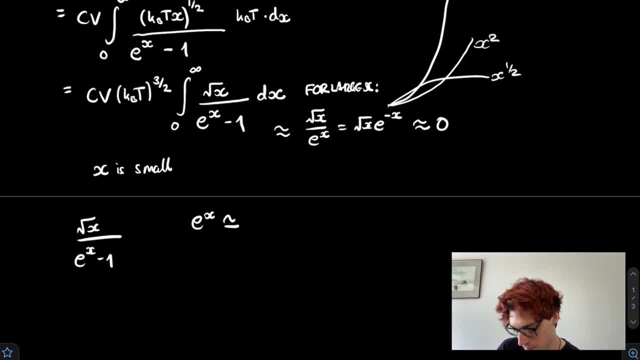 is approximately equal to the first order, one plus x. right there. Technically it will go on forever. it will go on. there'll be an x squared term, there'll be an x cubed term, so on and so forth. but because x is so small, it doesn't matter about these. like we can just look at the first. 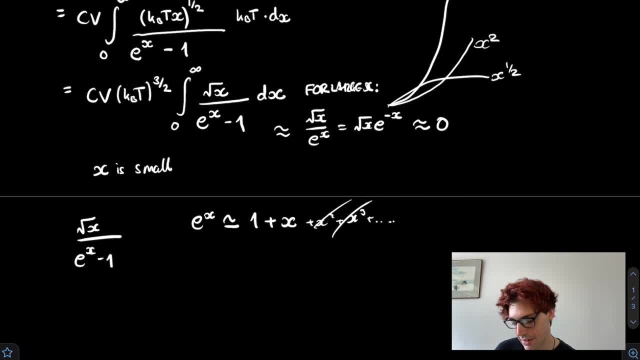 two, as that's the, that's kind of the only ones that are important for this. If e to the x is about one plus x, then we can see that e to the x minus one is basically about the same as x. so if we just subtract one from both sides, because of course these terms are so, so small- 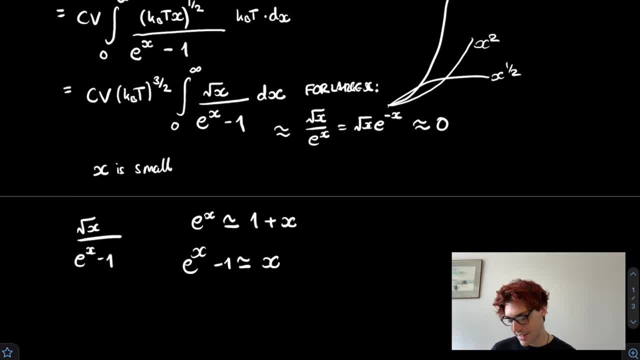 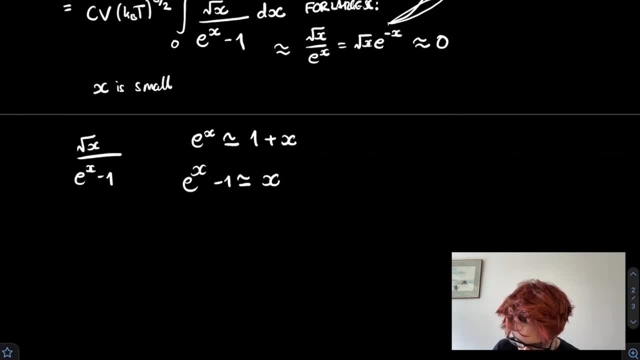 I'm going to rub them out because they are so small. e to the x minus one is basically x. So what happens to our integral here? Well, this, this equation: root x over e to the x minus one. what we said was that e to the x minus one is about x. so this will become root x over x. 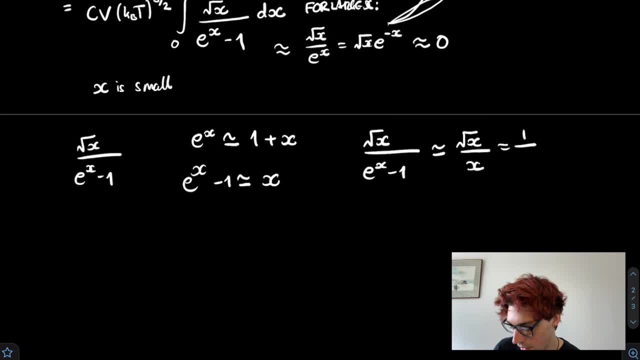 which is equal to one over root x. And again, what's going to happen when this is small? So again, when x is small, then you have one over root x, which, when you integrate over from naught to infinity, Then you can find that that is indeed a convergent integral. So this is fine. basically this: 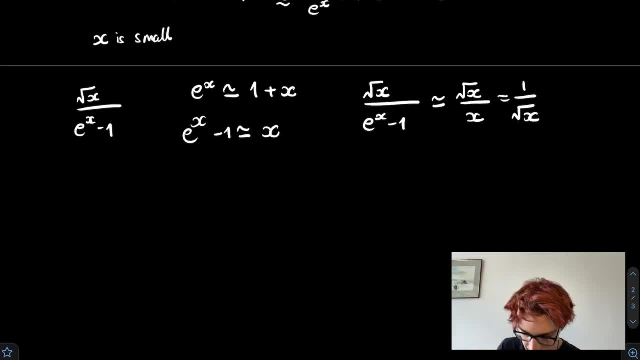 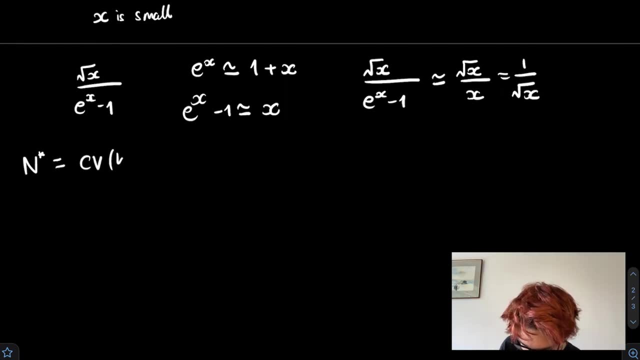 integral is completely fine, and let's just go ahead and rewrite it right there. So just a quick note: if this test doesn't work, if that you change, if you make x small and large, for either both cases, x doesn't converge, then you have a problem right there. So this is: 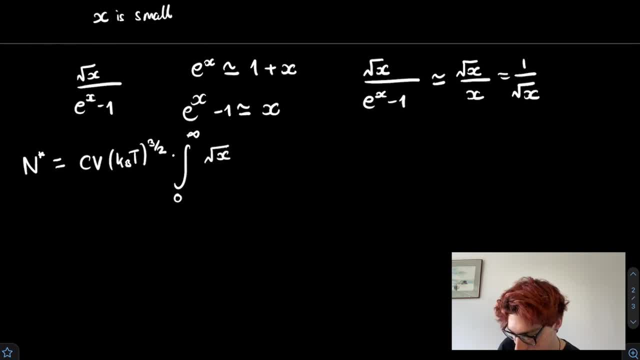 like a little mathematical trick, and if it doesn't pass, then it's not ideal, and then you can't get Bose-Einstein condensation. So there is our integral, Now this quantity. right here we've just shown that this is a. they are both convergent at both limits and therefore this is: 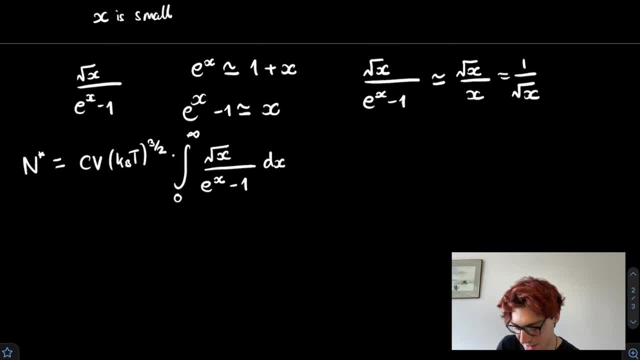 literally just a number. Like there's no, there's nothing physics-y going on right here, there's just a bunch of terms Inside. an integral like this is just a literal number right there. So what is this number? Well, this, just all this right here, is basically about 2.3.. Like, that's all that is. it's just a. 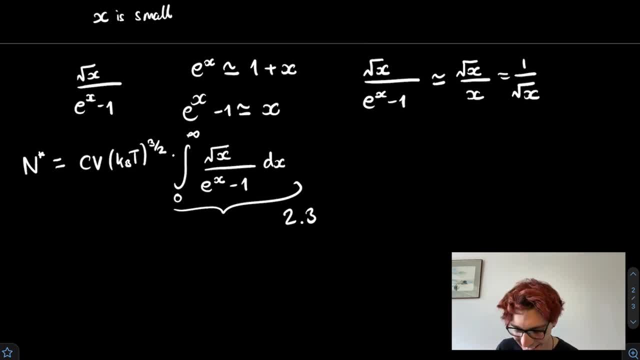 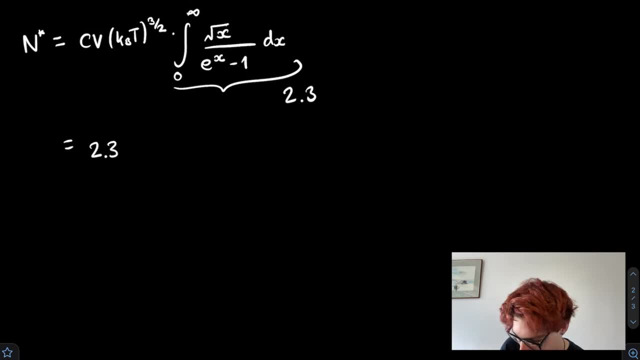 fancy way of writing 2.3, I guess, And so let's just go ahead and rewrite this in its much more simplistic form. So it's 2.3 multiplied by cv times kbt, to the power three over two. So that's n star. So let's just think about what we have actually. 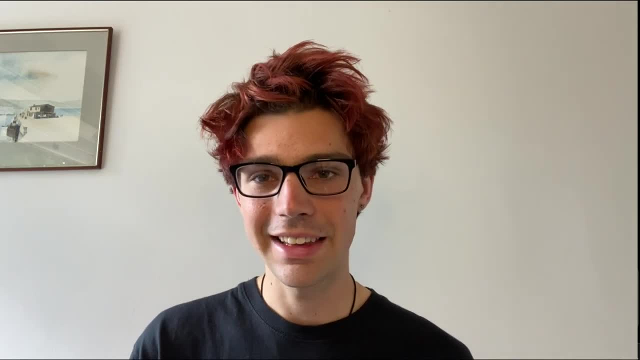 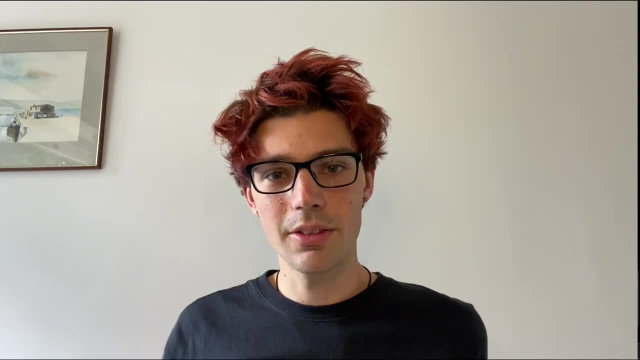 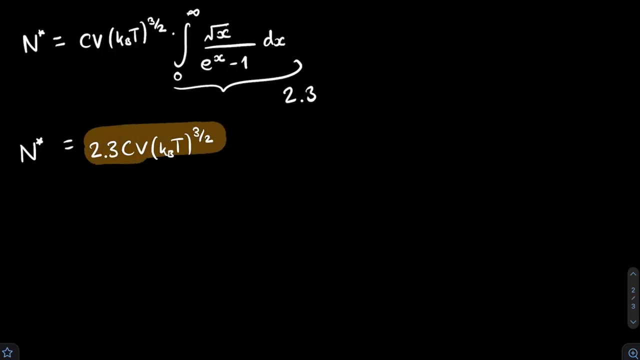 calculated for a moment. We have just shown that if we have a box and then we fill up our box full of bosons, we have just shown that there is literally just a number like this number right here. this is fixed. this doesn't really necessarily change anything, but this is a fixed number. So 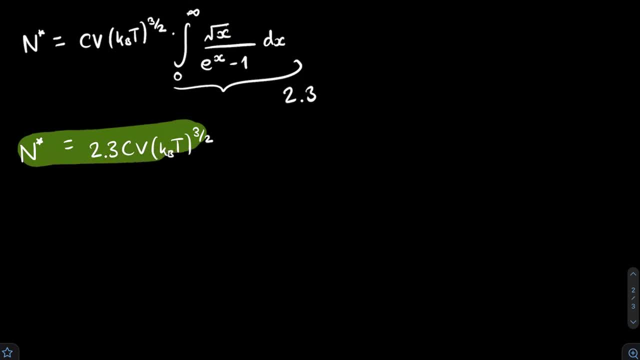 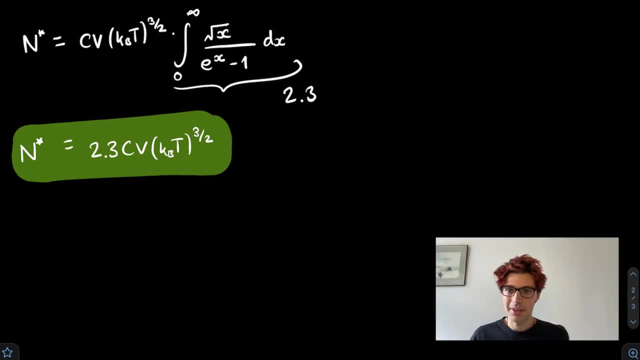 This is just a number of particles in a box of a certain volume at a certain temperature, And this is when we assume that the chemical potential is zero. So there is a slight problem here. This might look all right on the surface, but actually there is a slight problem with this analysis. 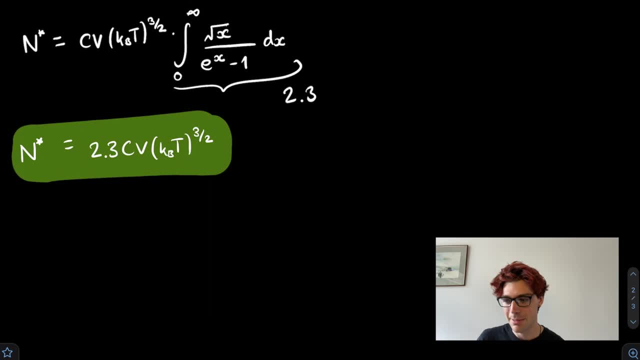 This is basically saying that at a certain temperature, you can't add any more particles to this box. So that's a bit weird, Like you know. imagine trying to add a particle to the box and just having it being like: no, you can't do this. 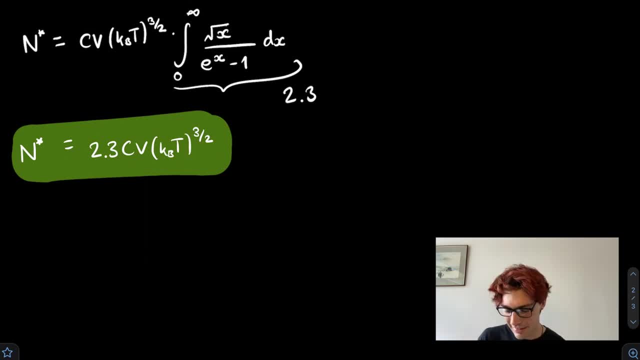 Like that's a bit weird, right? This is kind of what it's showing. You can only have this maximum number of particles in a box, And that would kind of imply that if you try to add another one, then there would just be some kind of weird force which would try and repel you from adding another particle to this. 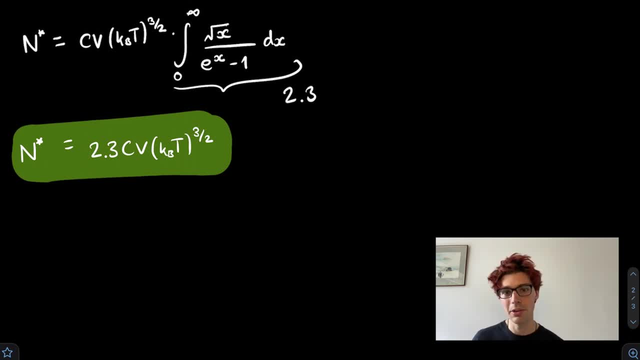 Because, remember, we are in the grand ensemble, Particles can flow in or out. It shouldn't be so that there is just this number, this constant number, that is, a maximum number of particles in the box. Conversely, this would also mean that if we were to lower the temperature of this box right here, so say we cool the box down. 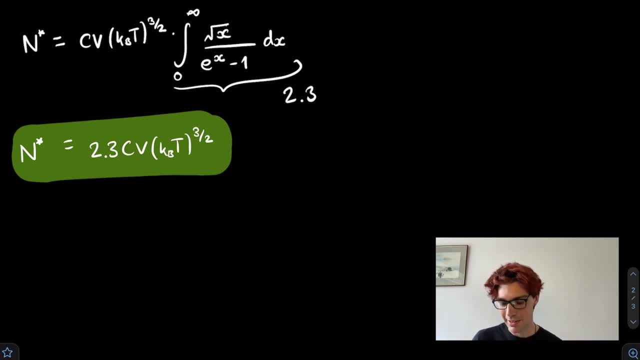 Does this mean that, like particles will gradually start disappearing from this box, like mysteriously vanishing from thin air? Like that makes no sense, No sense at all, like that is. that is really, really weird. So what is going on here? This is some kind of a paradox that we need to kind of explain, because this is very strange. 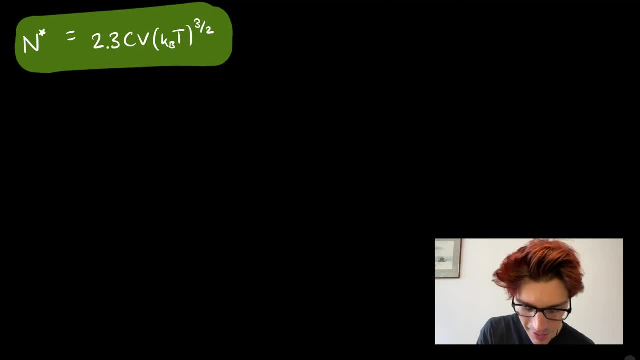 So the way we actually get around this paradox is to go back to our original graph that we had looking at the dispersion relation for our types of particles that we are considering. So if we go ahead and plot that right there, Then we get our parabola just like we have before our p squared over 2m parabola. 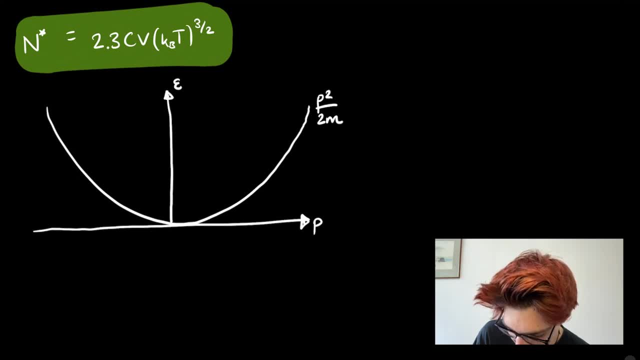 This is energy as a function of momentum And if you remember, the way in which we calculated this n star right here was just by summing over the different states and then multiplying by how many states, which is obviously the density of states thing. So just summing up. 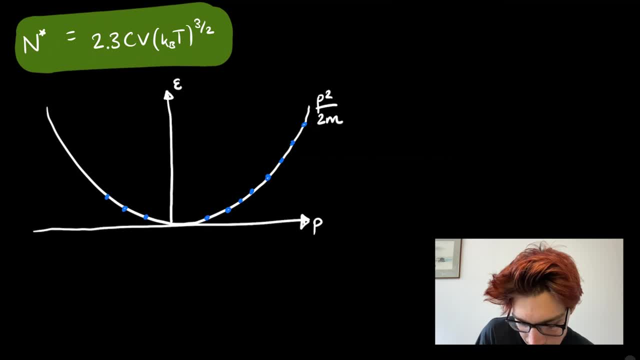 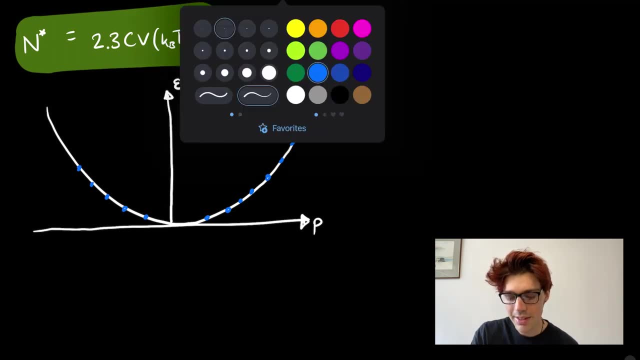 All these individual ones. We also did the ones for the negatives And yeah, we just kind of went up this like sort of infinite load of states. But there's one state that we didn't actually consider. It's this one right in the middle, right here. 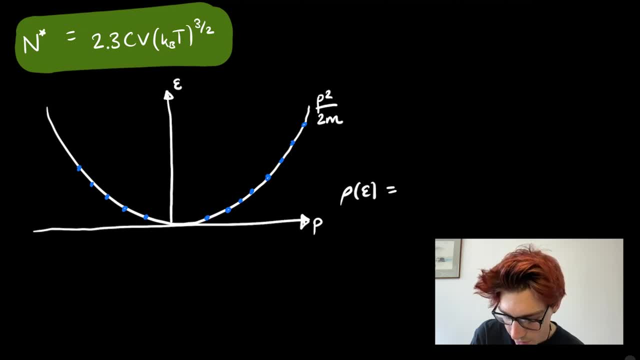 The density of states function does not accommodate for this right here. It only deals for states that are above zero, But it doesn't actually technically describe What's going on right at the center point right here, and basically what's going on is, rather than there being this kind of fixed number, of course the same number of particles will still be there from when you start sort of cooling the gas. 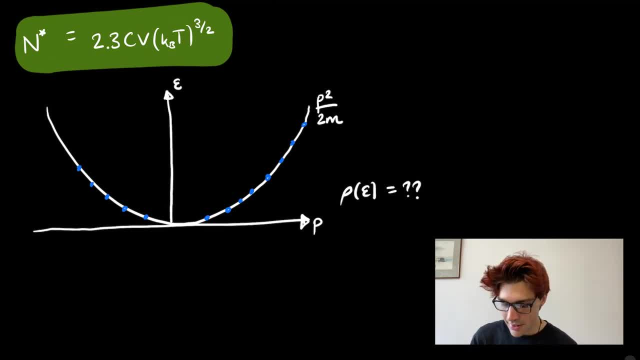 So the thing that's happening is that particles are basically starting to all pile up in this state right here. So all the extra ones, all of the extra particles that are not n star- so you have n star particles that are not sort of there, but then you have all these extra ones right here. all these extra ones are all piling up in the middle. all in this kind of p equals zero dispersion curve, right here. 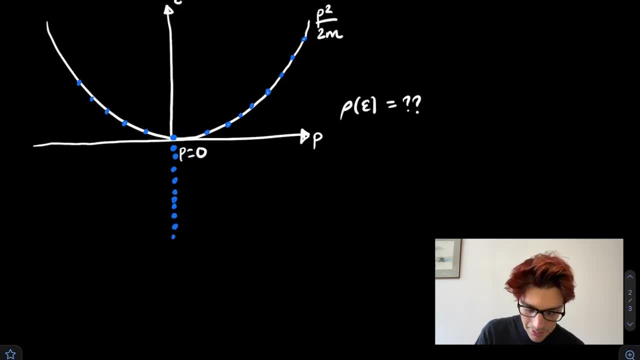 Now what's going to happen when we start piling up loads and loads and loads of these particles? there's going to be way more of these particles in this part on all- in this kind of p equals zero part of the dispersion curve- than all of these right here. 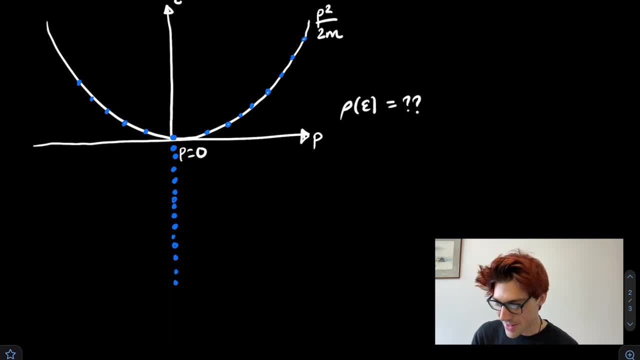 There's going to be way, way, way more and eventually you're going to start having ridiculously high numbers, and that, right, there is what the Bose-Einstein condensation is going to be, And what that condensation is. it's basically all these particles in the ground state of this dispersion curve. 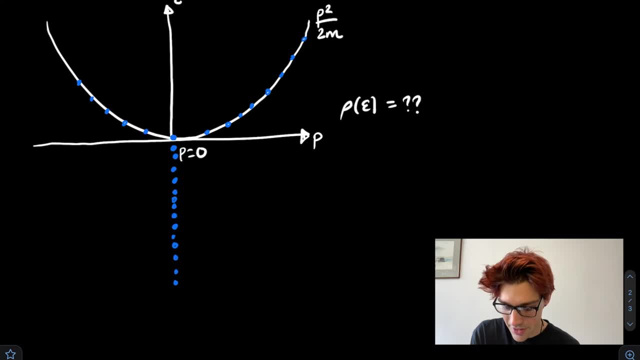 So they've all got p equals zero, they're all. all their wave functions are kind of infinitely spread out, or not technically infinitely, but like really really spread out throughout all the space And they're just all kind of there. So what is it that we're talking about exactly? 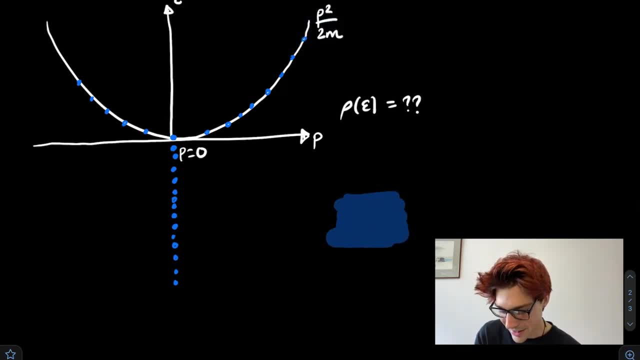 We're just kind of talking this kind of ghostly kind of haze that's just around. So it's this really weird idea, like they're just all kind of floating around, I guess. but they're, they've got zero energy and their position is not very well described because their momentum is zero. 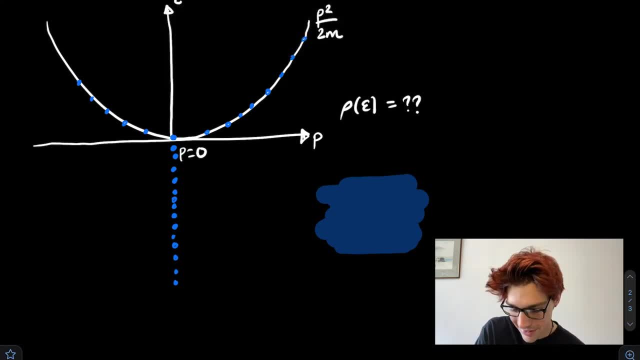 So their position according to the thermal wavelength lambda equals h over p. like their wavelength is just spread out, So We can't accurately determine where they are, and that is what it is. It's crazy that this is even a thing. 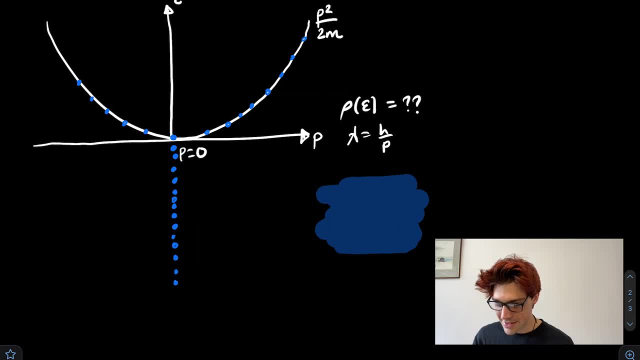 That is what a Bose-Einstein condensate actually is. It's an infinite load of plane waves just hovering around and you can get some really cool effects from the Bose-Einstein condensation. And we're going to talk about just a few in right a moment. but what I just maybe wanted to touch upon, this kind of transition between 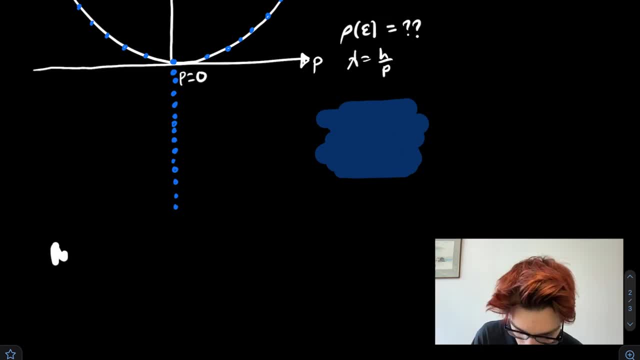 Bose-Einstein condensate. so from from normal gas, from like normal gas behavior going to Bose-Einstein condensation. This is an example of something that's a little bit more general in physics and something I'm going to hopefully touch upon. 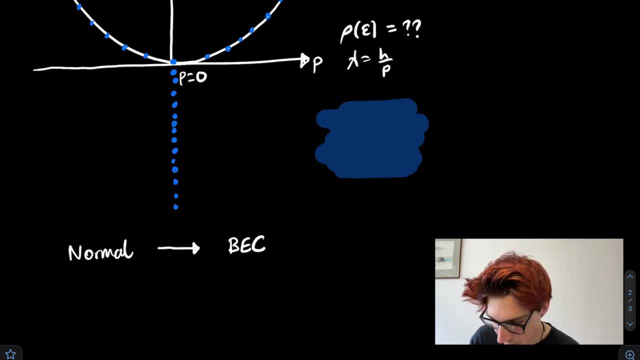 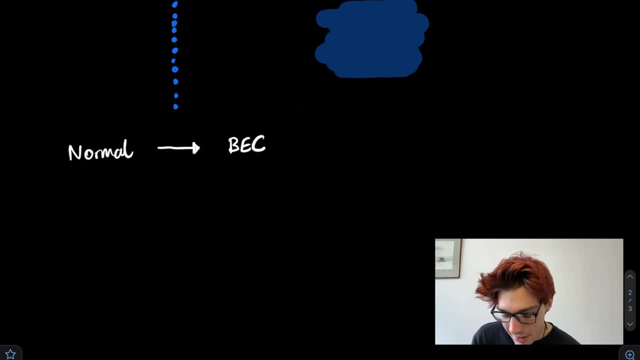 This is an example of a phase transition, And what this is. a phase transition is basically something where you have this one kind of kind of state of a system, this kind of normal state. If we reduce temperature or anything else, then you end up in this kind of different state, right here. 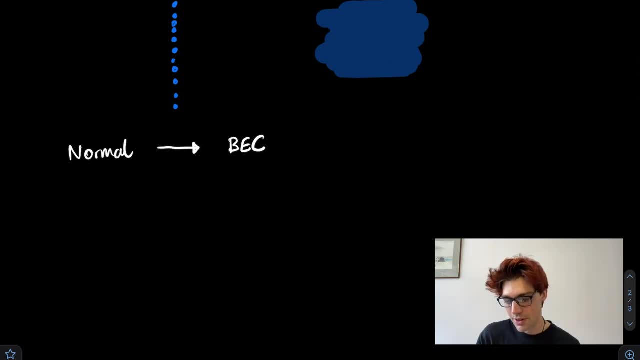 Like very suddenly, there's no real kind of smooth transition, It's a very quick kind of jump And in fact if we just draw a graph of what of basically temperature and sort of the number of particles that appear in like the Bose-Einstein condensate, so this will be like: 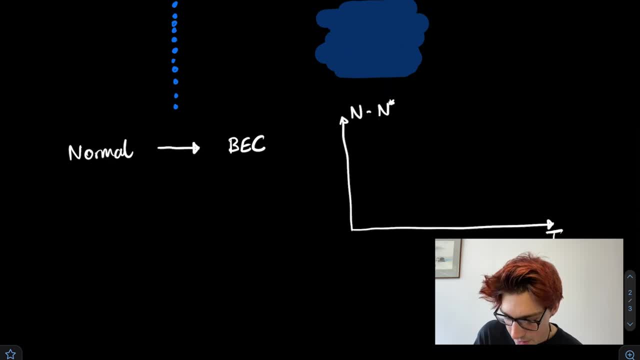 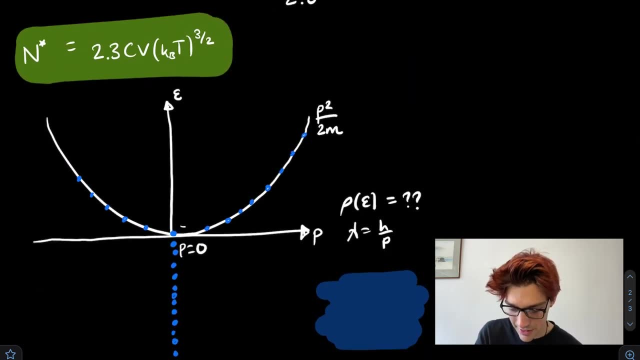 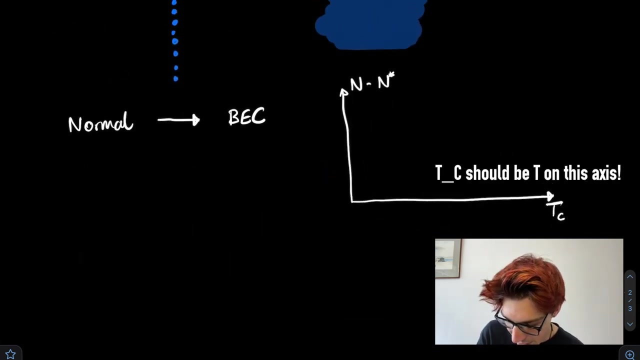 n minus n-star, where n is the total number of particles in the gas And n-star is this number that is not in the condensate. This is the number that's kind of being occupied in this part of the graph. So if we, if we plot that, then as we cool the temperature, of course we have nothing for ages and ages and ages. 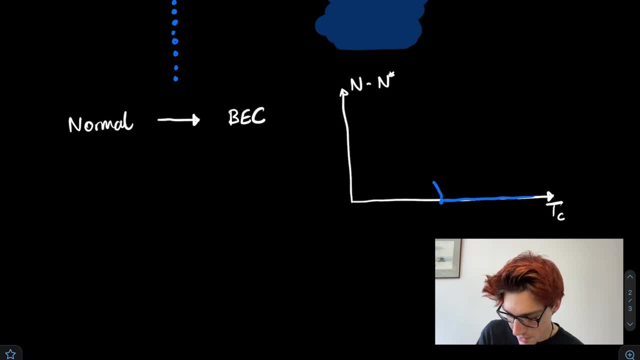 And then suddenly, at this critical temperature, we get this light, this jump, where you suddenly start getting particles in the condensate right here. So like particles just start piling up at this very like sudden critical temperature, which is very weird, because not a lot of things in physics really behave like that suddenly. but that is what is. 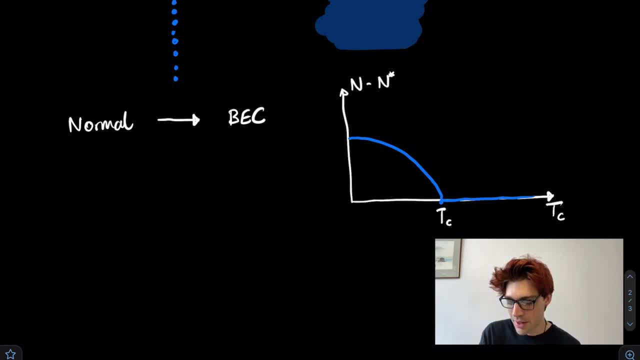 actually happening. You're suddenly getting this jump from nothing to basically Bose-Einstein condensation at this critical temperature. So this is what I just wanted to touch upon is that it's a more general example of a phase transition. So one last thing about Bose-Einstein condensates. 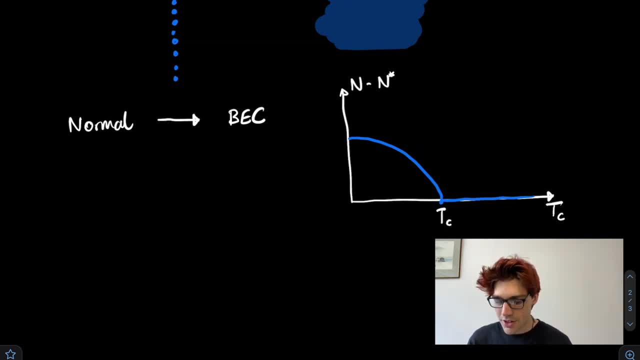 is that not all of them, but some of them- show a phenomenon called superfluidity. Now, superfluidity is really, really cool. It's almost ghost-like. Imagine this kind of ghostly phantom haze That is able to kind of defy gravity and just sort of not quite know where in space it is. 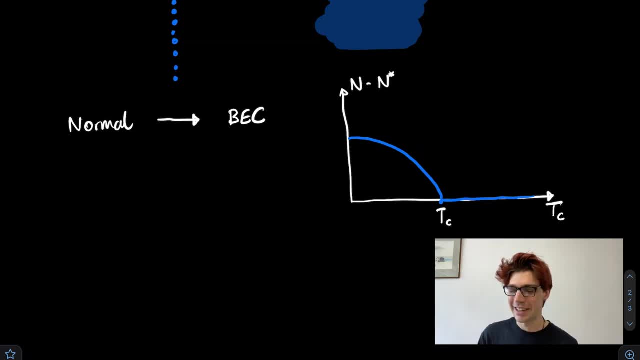 That's basically what superfluidity is and it's really really cool. Most Bose-Einstein's condensates show superfluidity. Basically, the physical thing that defines it is: with the viscosity of the fluid, mu is equal to zero. There is no viscous force on this fluid. It's basically 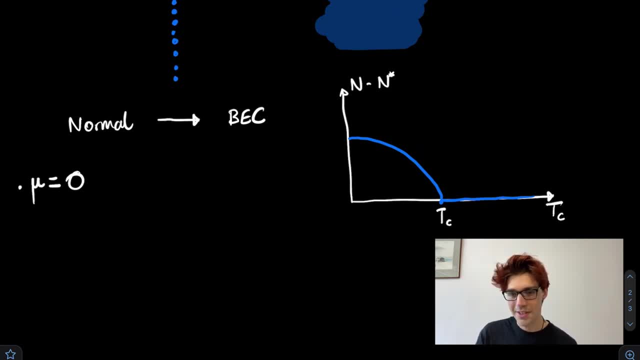 free to sort of run along a surface infinitely without being slowed down, Because in a normal fluid there are shear forces, which is basically viscosity. They are what slows the fluid down. That's what kind of defines a fluid, Whereas a superfluid, the viscosity is just flat out zero. 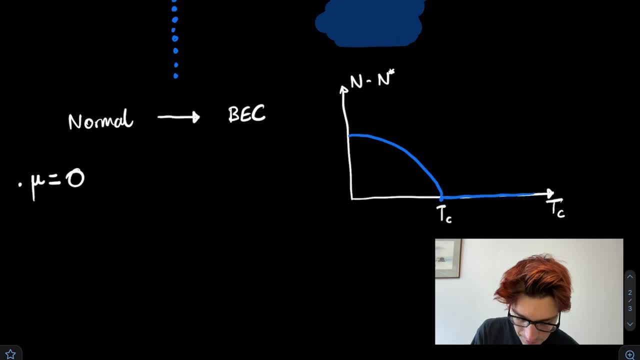 So just to illustrate what I mean, I'm gonna draw sort of a jug. So here's our jug, if you like, And we're gonna fill this jug up with some Bose-Einstein condensate. And obviously this jug is kind of sat on like a table and, you know, it might be sort of in a 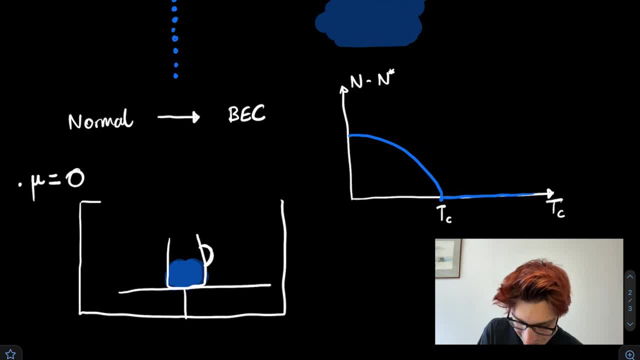 room or something right there, Then the thing that's gonna happen once you put this Bose-Einstein condensate in a jug, then it will actually kind of basically run up the walls and then just kind of like basically just go all the way around the walls, just like this, And then it will just sort 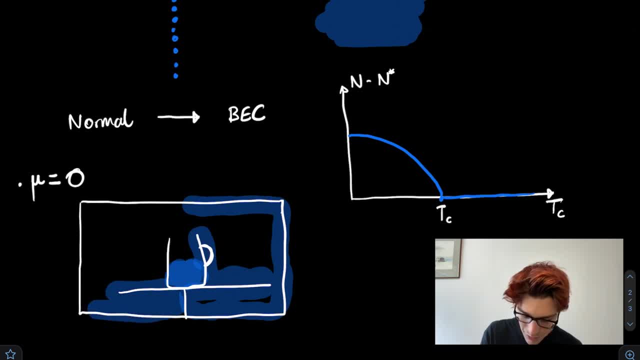 of flow to coat the walls, as if there's no force stopping it, Which there isn't. There is no force stopping this, this Bose-Einstein condensate, from flowing all the way around the table and then just going all the way along the floor and then up the walls and then up on the ceiling. right there It's. 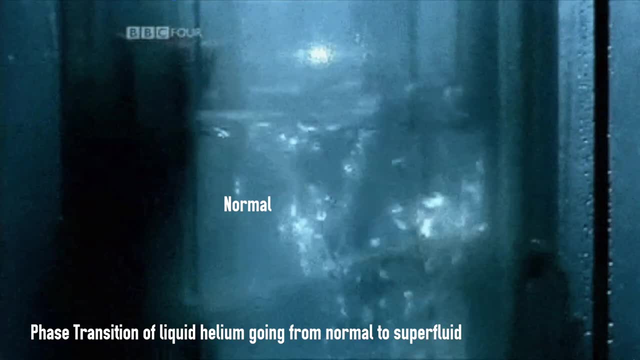 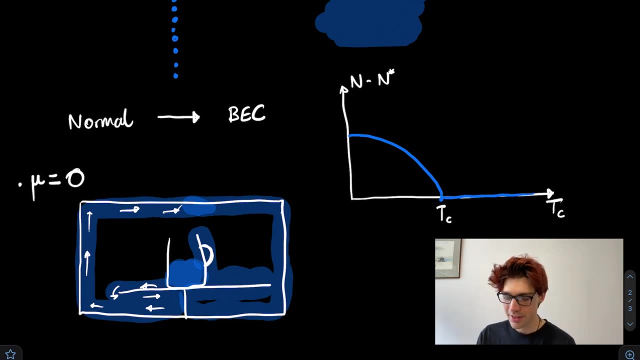 really cool, And that is basically what superfluidity is Basically. no force is stopping the fluid from going across the surface. The condition that a Bose-Einstein condensate needs to have for it to be superfluid is basically known as the Landau. 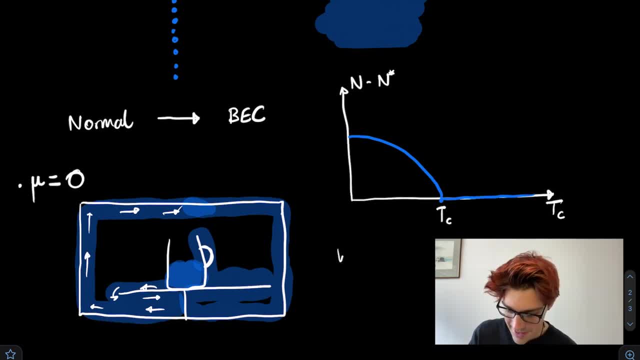 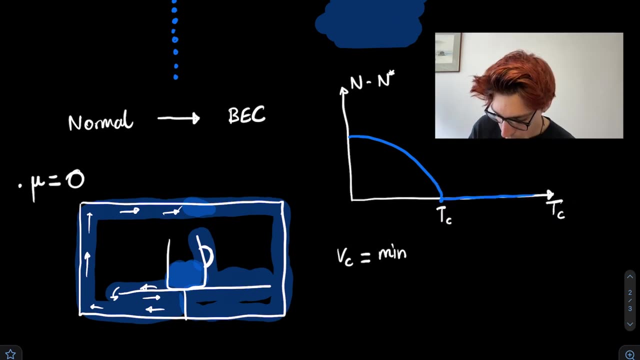 criterion. And what the Landau criterion says is that there is a critical velocity, vc, below which a fluid will move like a superfluid, And it's basically defined by the minimum of the energy divided by the momentum. right there, That's all a little bit vague. I'll just elaborate. 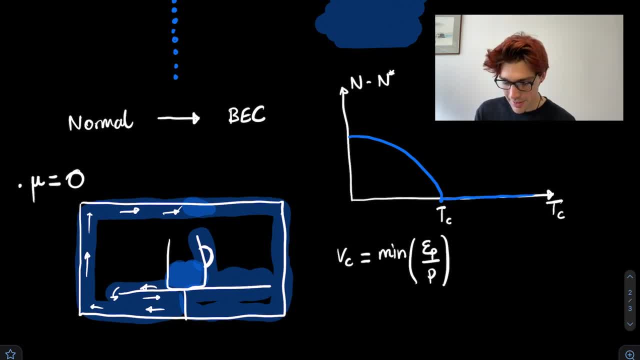 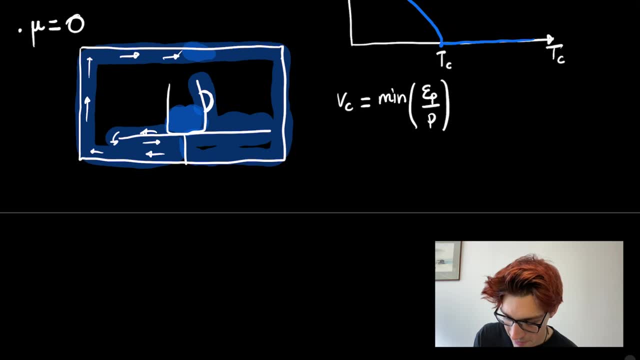 on what that means For a normal fluid. so like this one we've just been considering. right here, it actually turns out that you can't have superfluidity, Because if we plot the dispersion curve, then what's the minimum of this kind of ratio right here? Well, the minimum vp is: 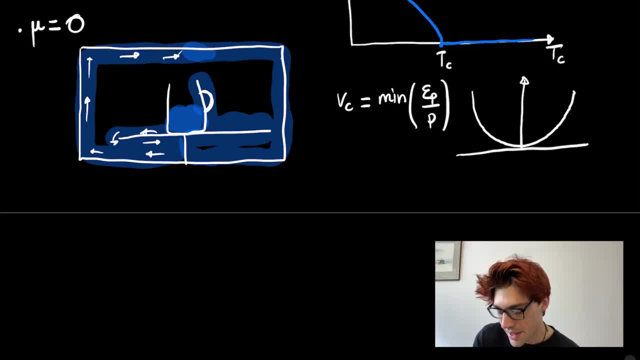 going to be here, And if we divide by p it's not going to really make any difference. So it's just going to be p squared over 2m, all divided by p, which is just p over 2m, And the minimum of that is still zero. 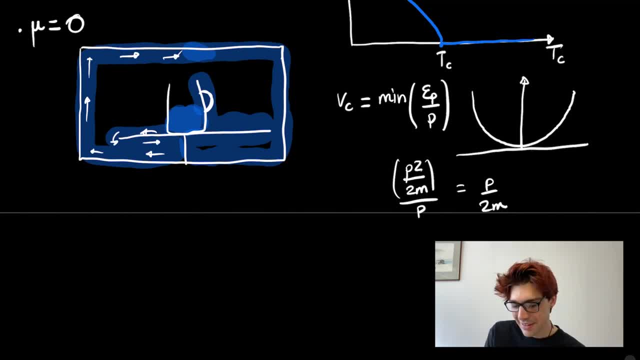 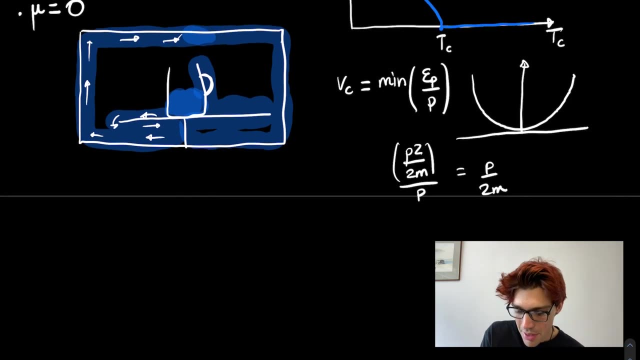 right there. Since the critical velocity below which has to be satisfied, and since in this case there is no critical velocity, it's just zero, then in this case, with this dispersion relation, you can't actually have a superfluid. But I'll show you an example of a dispersion curve which can be superfluid. 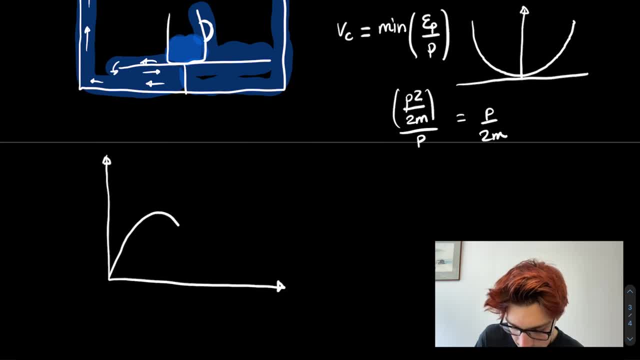 So say, we have this graph right here that goes something like this: So we have this kind of minimum right here, And if you analyse the curve, then you take the ratio of ep over p at each point, then you'll find that at this point 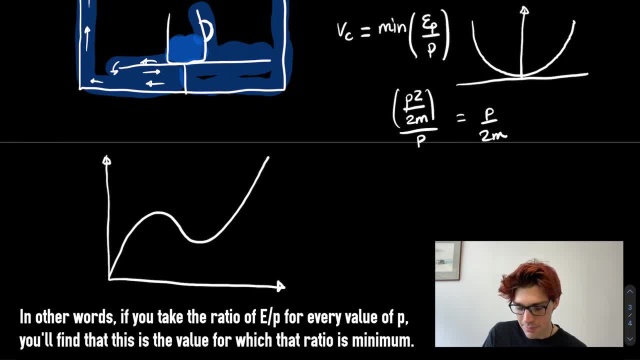 right here. there is a minimum in that And this minimum is non-zero, like this velocity minimum. You can kind of see from the graph, it's non-zero And yeah, this right here is the critical velocity And anything below this velocity which you'd have to know, the exact equation of this curve. 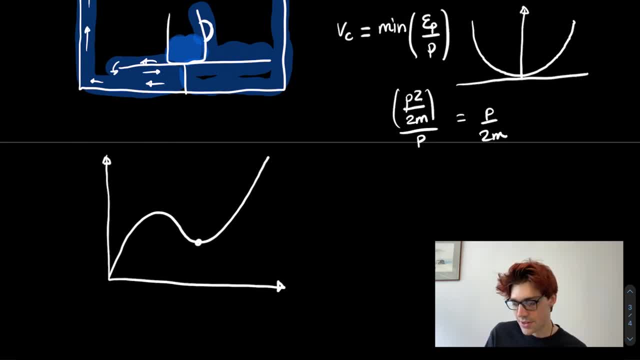 but anything below this velocity you will have superfluid behaviour. Above the velocity then it just behaves like a normal fluid, But below the superfluid, below this velocity, then you basically get superfluid behaviour. And yeah, it's really cool. 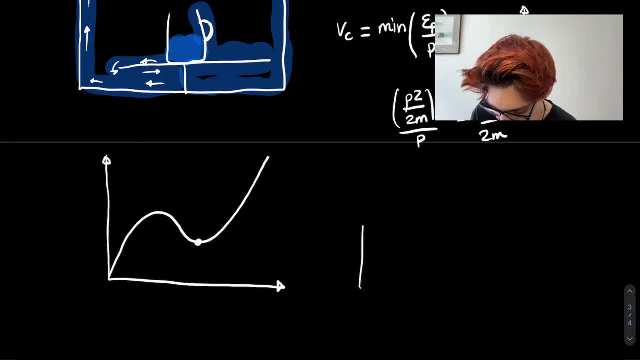 One other way to look at it is by considering: say, you've got this like little bowl and inside this bowl you have a Bose-Einstein condenser, And then you have a spoon which you dump into the bowl right there. Now, what do you normally expect with a fluid? Well, 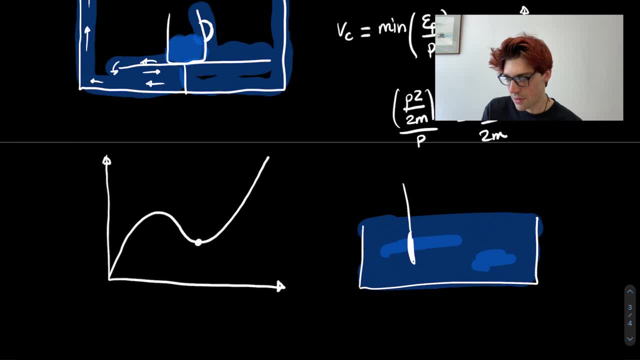 you normally expect, as you move the spoon through the bowl, the fluid to kind of drag along with it And the fluid to sort of, you know, create some kind of like disturbance. there's gonna be some sort of sheer force, But of course, with 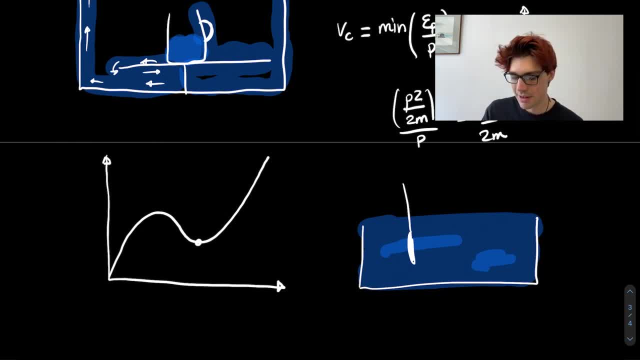 a superfluid, then there is no sheer forces, there is zero, And what you'll actually find is when you move the spoon through, then you'll find the fluid won't change, Which is a very ghostly kind of weird thing to experience, Like if you- I- had a. 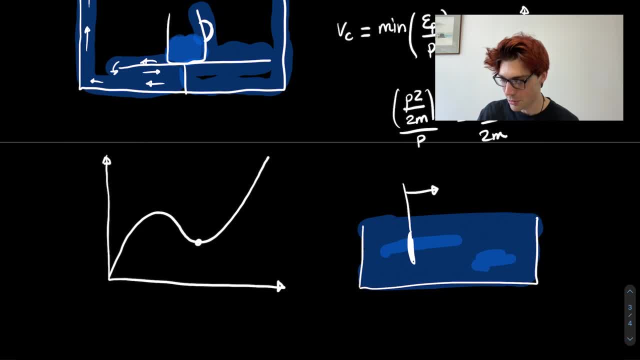 sort of imagine moving a, moving something through what appears to be a fluid. then there will be no sort of disturbance from in the fluid up till the critical velocity, after which, yes, you'll experience turbulence and flow. so, basically, what is the maximum velocity you have to drag the spoon? 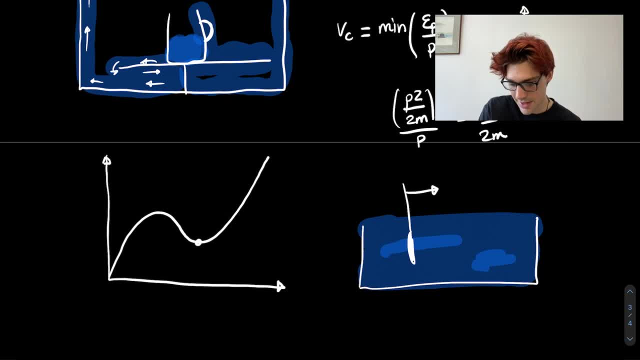 through in order to not experience that. well, that's vc, that's the critical velocity, and that's another way of looking at basically what that means, and that is basically super fluidity in a nutshell. so, yeah, i hope that was an interesting video. guys, i find this stuff really really cool. 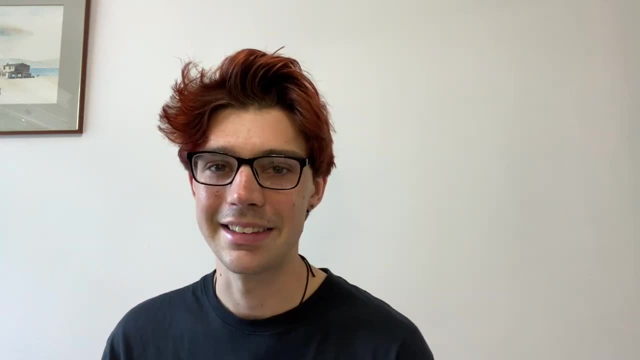 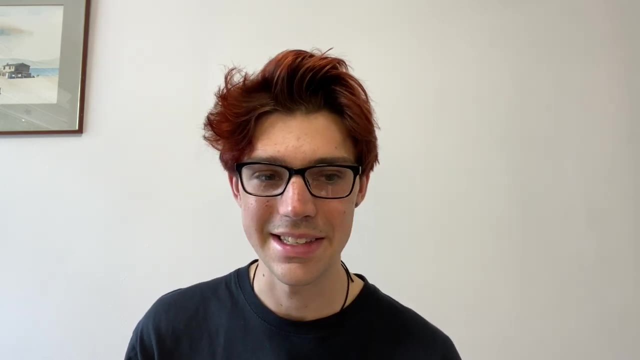 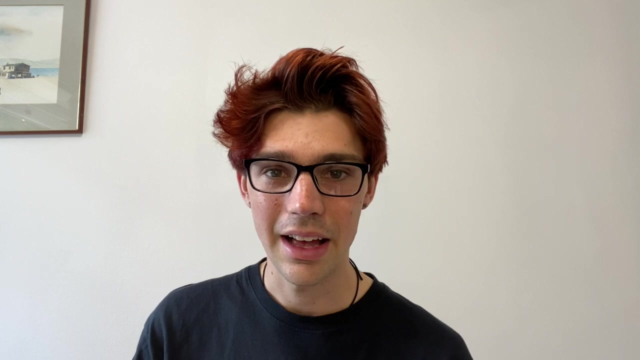 i think it's amazing that there's a whole nother state of matter that none of us are really that aware of, and it can kind of sometimes go up walls, which is amazing and very, very weird. just more of quantum weirdness, i suppose. so yeah, in the next video we're going to be having a 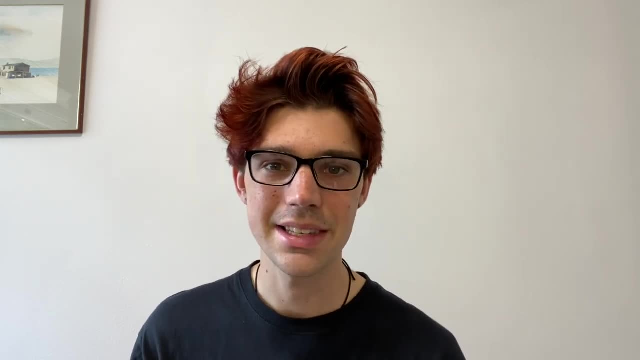 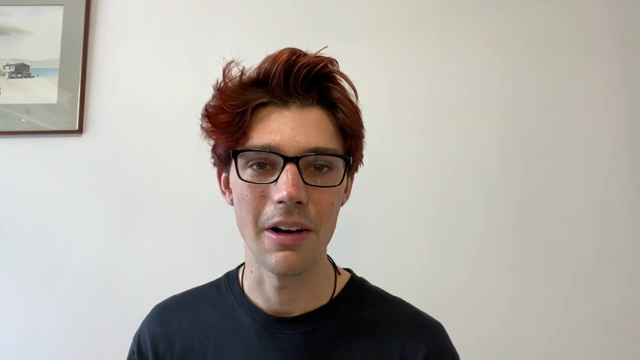 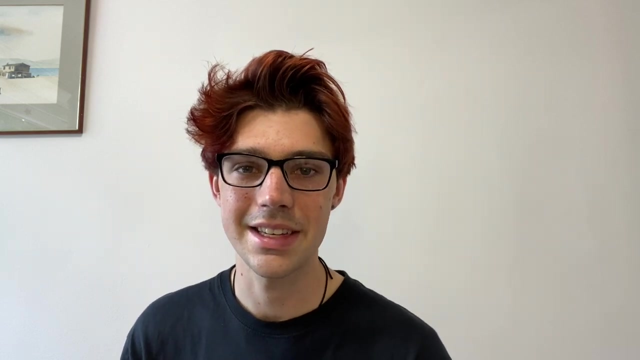 look at fermions. We've had a look at bosons and now we're going to have a look at fermions and we're going to be looking at how fermions are a very good model to describe most metals and how you can actually do things like solid- a lot of the solid state physics and semiconductor.